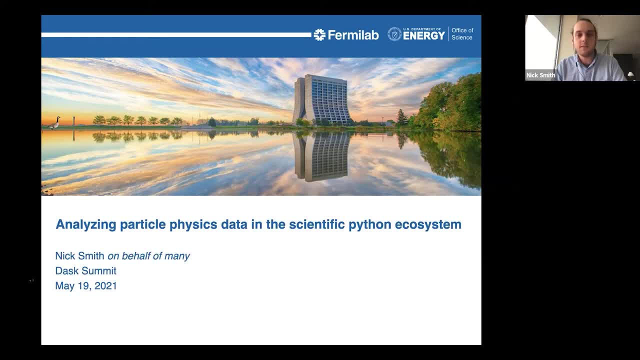 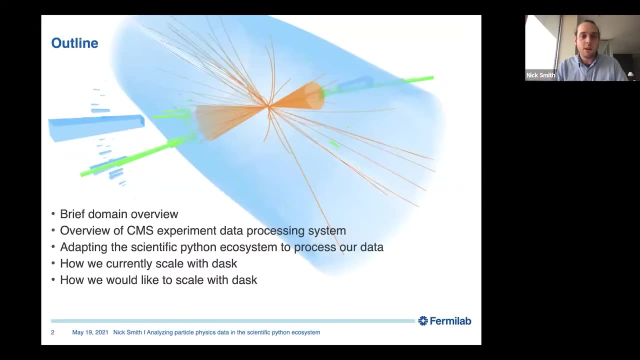 about how we've approached our data analysis task with the ecosystem that you're all familiar with, And we- I mean very many people like too many to put on the slide. So let's get started. What is I'm just going to give like a brief domain overview. try to make it interesting and not too. 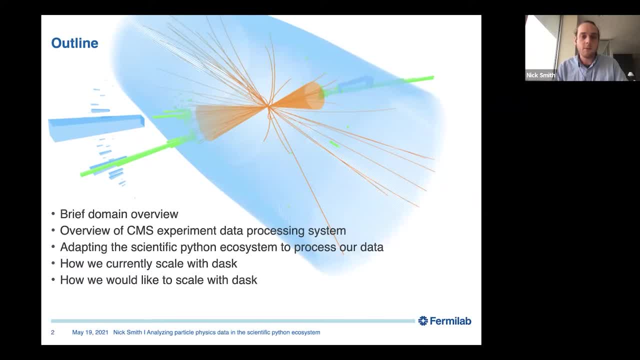 technical Kind of a detailed overview of exactly how we do our data processing- you know, the full data processing- And then I'll narrow in on the analysis step, which is sort of this last step where scientific Python tools such as you know. 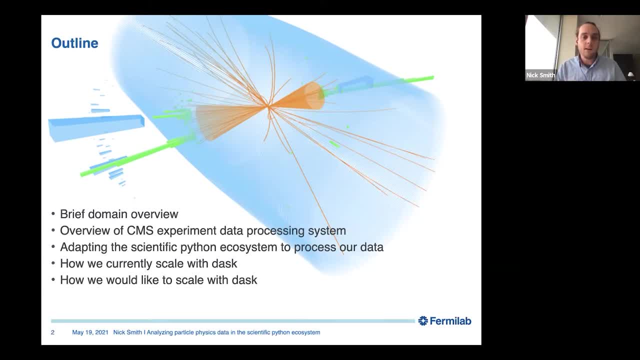 like the Dask ecosystem starts to become applicable, And then I would dive into, like, specifically, how we adapted scientific Python to make it usable for our data and how we scale it with Dask, And then then finally give an outlook on what we think we could improve with our, with our system, And I hope people sort of take away, you know. 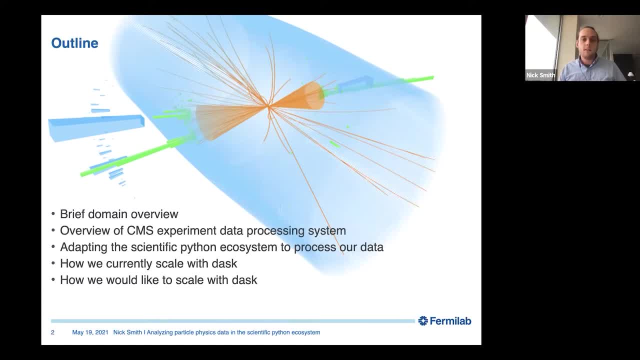 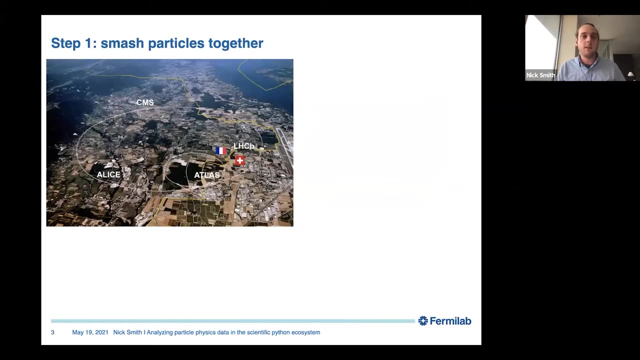 from this, things that may be familiar in their, in their problem domain, that they might be able to lift and or collaborate with. Okay, So if I want to describe particle physics in three steps, I'll try to do that. Step one: 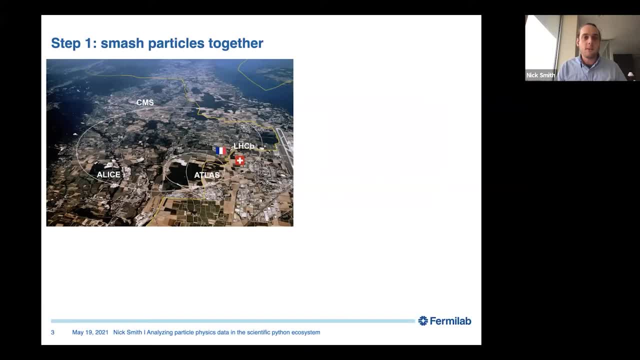 you smash particles together. So, as mentioned, I work on CMS, which is one of the four LHC experiments, and the Large Hadron Collider is this big ring underground between Geneva and France, And it's the latest in the long line. There was one outside of Chicago, There's one in. 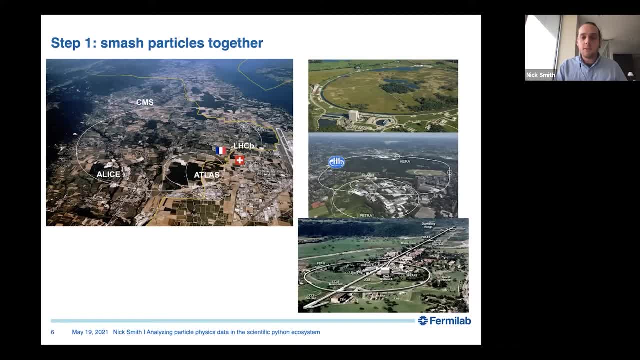 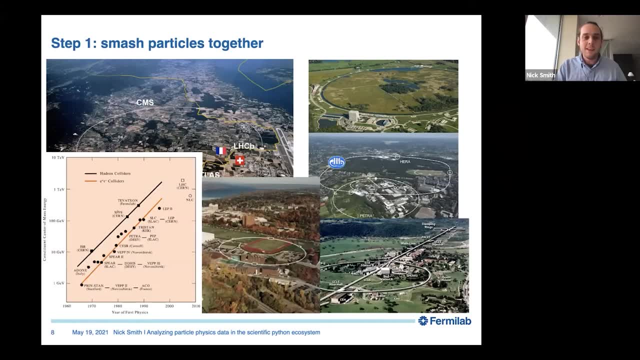 Hamburg, There's one in I don't know New York. There's one in New York, There's one in New York out at Stanford. this is actually a linear accelerator instead of a rain. here's one underneath a football field at Cornell and just basically. you know in the past, say 50. 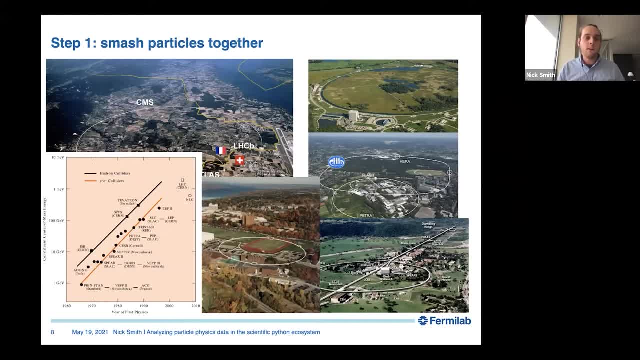 years or so, there's just been this exponential growth of center of mass energy. so how hard we smash them together and each one brings a new information about fundamental particles. and yeah, so it's been growing exponentially, you know in this graph. but you know, the history goes. 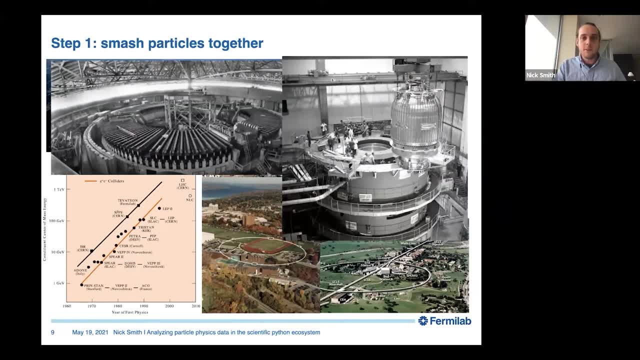 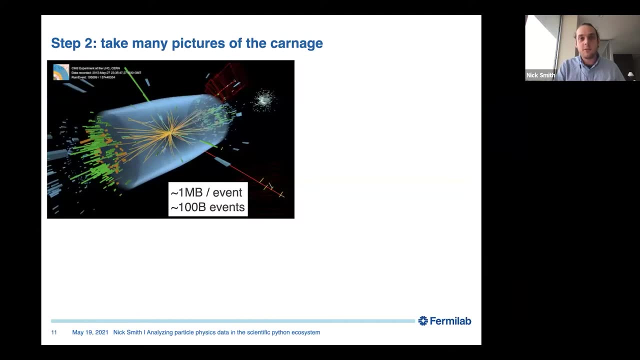 back further. there were here's some photos of some that were in black and white, so it gives you an idea how old they are, and the very first one is actually could fit in the palm of your hand. it's this little cyclotron built in 1930.. Okay, so step two: take pictures of the carnage. 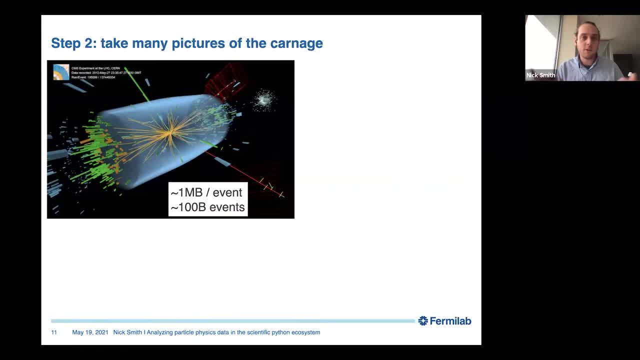 my experiment takes one megabyte pictures per collision event and we collected about about 100 billion events so far, so that's about 100 petabytes of data, raw data, um. previous experiments, such as the one at Fermilab, collected a little bit smaller data and a lot. 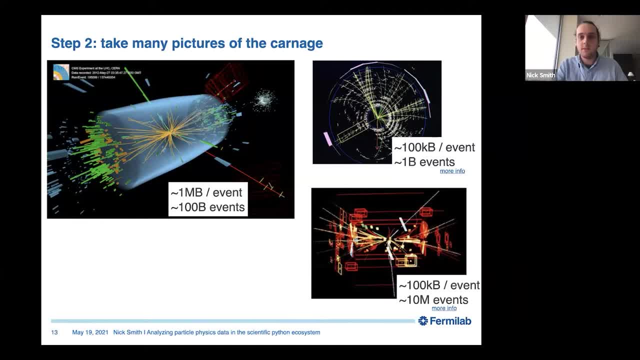 smaller events and then, if you go back even further in time, this is an event display from from, you know, the early 80s, where they only collected 10 million events. so basically, there's been a similar exponential growth in the number of rows collected, or particle, you know, collision. 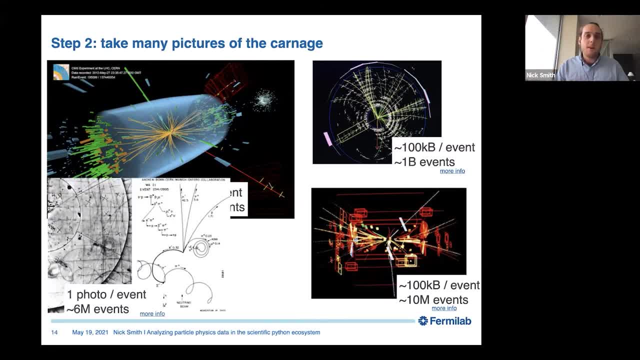 events. and you know, if you go all the way back to these- uh, these first bubble changers at chambers, it was literally a lot of data that was collected. and then you go back even further in time. this is an event display from, you know, the early 80s, where they only collected 10 million events. so basically, 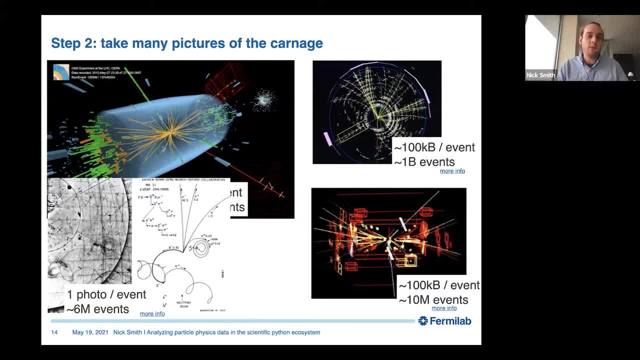 a photo. you took a photo of the particle trajectories as they went through a special bubble chamber and you sort of hand analyzed them and figured out the trajectories of the outgoing particles, and what kind of particles, and their kinematics. it's kind of amazing actually that the six million such photos were hand analyzed. so big data used to be, I think, a lot harder than it. 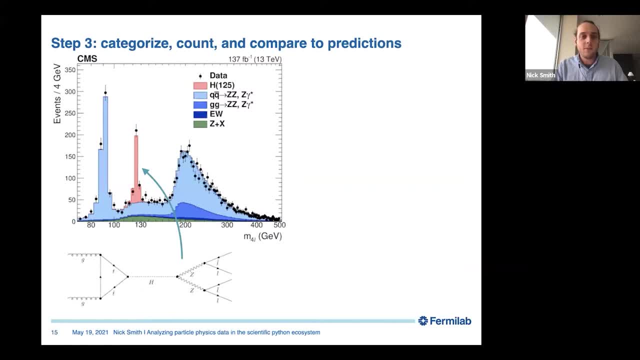 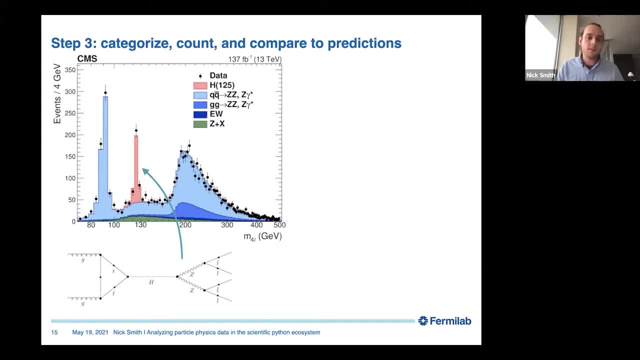 you know these funny diagrams correspond to actual math that predict rates of different types of events. and then you look for you know, basically rate excesses above what you knew at the time and if you're lucky you find something like you know, the higgs boson here, the top quark here. 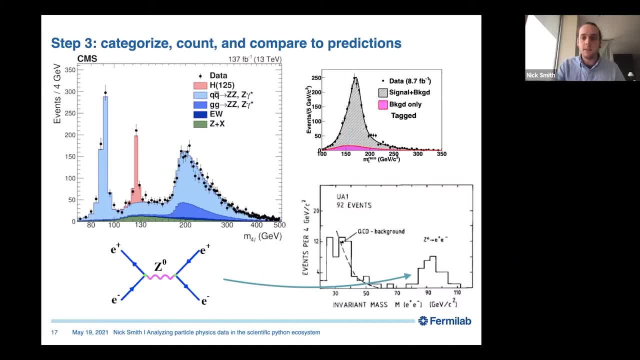 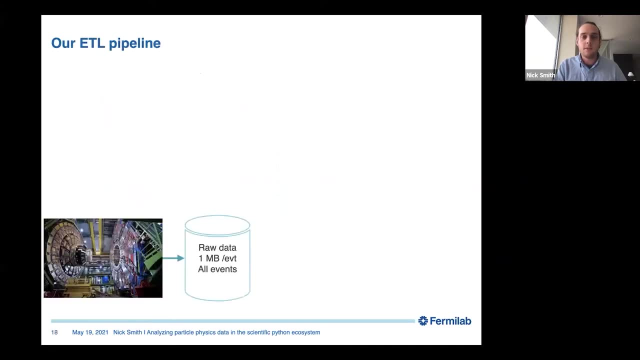 or the z boson. um, you know, way back in the 80s- and this is actually, you know, one of the you know 10 million event plots that turned into only maybe like a handful. so you can see there's a lot of filtering going on and presumably there's a lot of work to 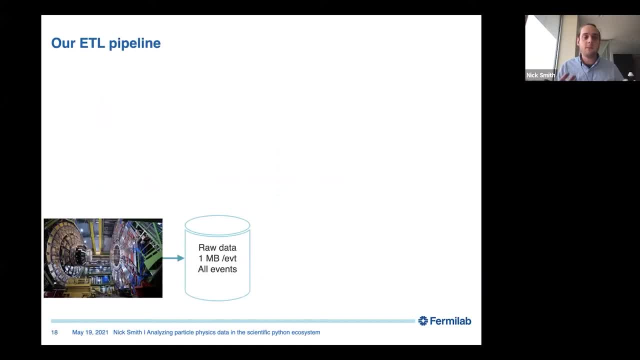 to, you know, compact this raw data into something that actually can be put in a plot, and indeed it is right so. we have, you know, one megabyte event raw data. we have 100 billion events, that's 100 petabytes. we can't analyze that in a day. we also have all the simulations that correspond to. 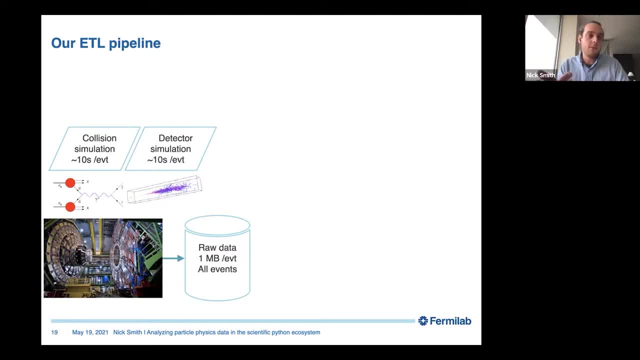 and we do like detailed uh simulations both of the both of the collision itself and then the detector simulation as the outgoing particles traverse our detector material and how they interact with matter and how we actually detect what happened, and we combine those into this reconstruction step and then write that out, and so now we have this experiment managed. 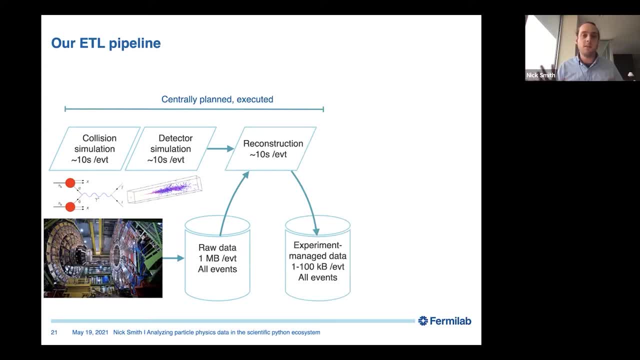 data that's, maybe you know, one to 100 kilobytes per event, depending on you know what information you're saving and you're still saving all the data. this is all something that's centrally planned and executed by the experiment and, you know, has been developed with custom software over you know a few. 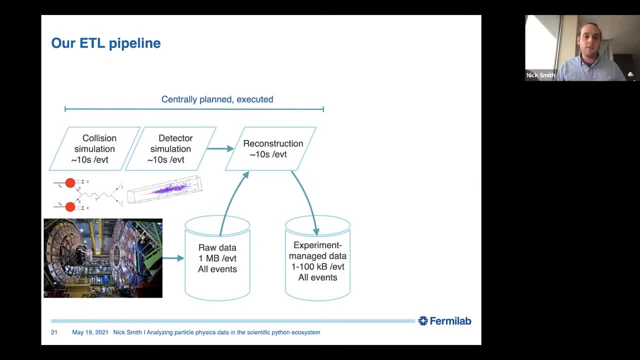 decades now and you know it's executed over a big grid. but after you get through all that, you still actually have to do some physics with this. you know this reconstructed data, these, you know- analyzed pictures, and so that's when you get to this end user analyst stage, where you know it's. 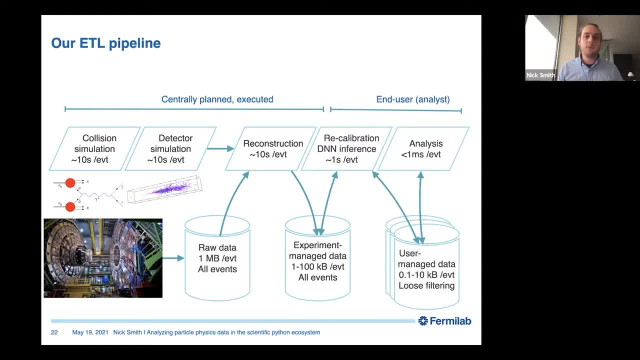 actually individual people, individual groups of people from many different universities looking at this data, looking at their piece of the data, trying to understand what happened, what you know what kind of topologies they're interested in, and so they have to do things like recalibrations, maybe run some deep neural network inference. you know things that are. 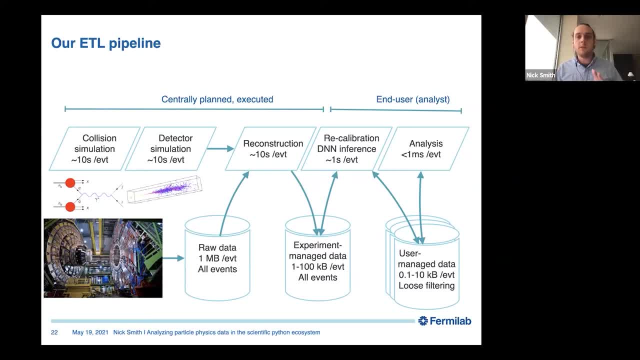 more on the scale of one second per event, and they probably don't have to do it for all events. they can probably do some- you know- early filtering to to reduce the amount of time they have to spend and then you know, you end up with this. you know, maybe user managed intermediate data with you know. 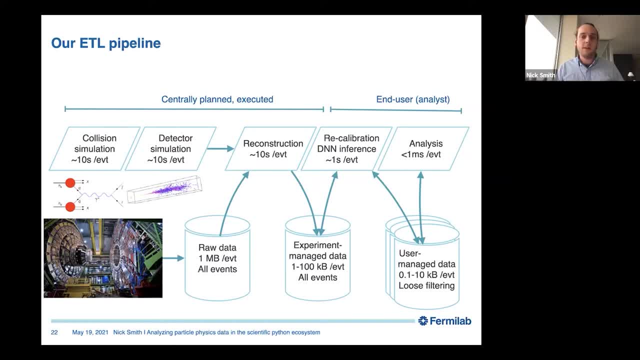 some like 0.1 to 10 kilobytes per event and maybe you know a tenth as much data. so now you're you. if you, if you multiply that together, you're in the kind of terabyte range now. so terabytes is something i think people in this conference are a bit more familiar with, and that's where we start. 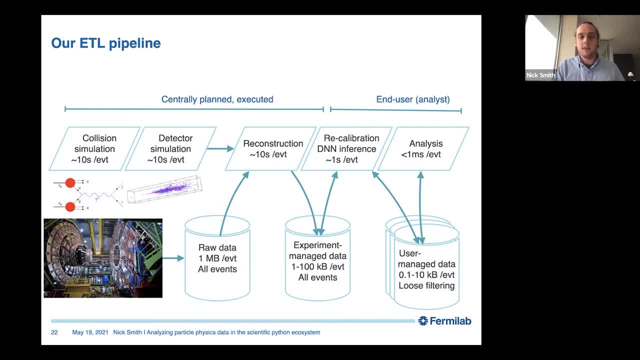 to see, um, the opportunity right, uh, to issue our sort of custom, you know, uh, boilerplate for something a little bit more modern. but of course, you know, sometimes people might need to do some checks of the earlier reconstruction maybe. uh, you know, we, when we first turned this on, we, 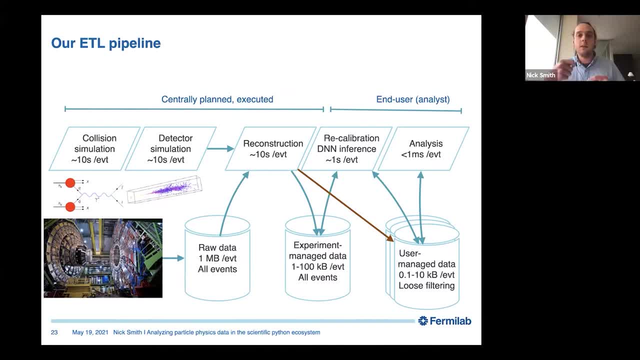 actually know 100 how it was going to work. you know you have to tune your algorithms, right, you have to, you know, do some data quality checks and so, as time progresses, right you, you sort of move that, those early checks and those early uh calibrations into the centrally main software. 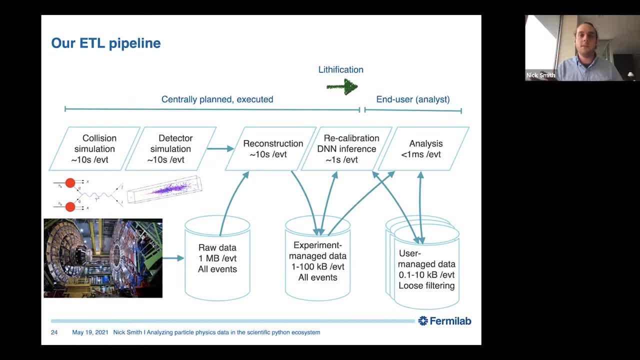 and i like this term that comes from the software community: lithification- right, you, you have this like mess of different approaches and you kind of settle on one and you bake it into the software and leaving, you know, less work for the end user. and so now you know, after almost a 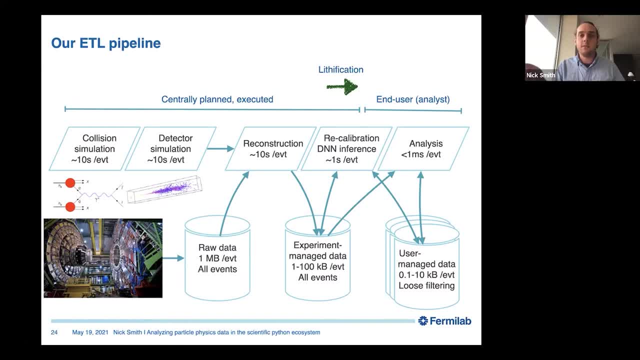 decade of running, we start to have these experiment managed data that's already, you know, pretty much ready to go for analysis, which makes it even nicer to start looking at these other tools, and so, yeah, i'll focus basically on this this last part. uh, one thing that's happened quite 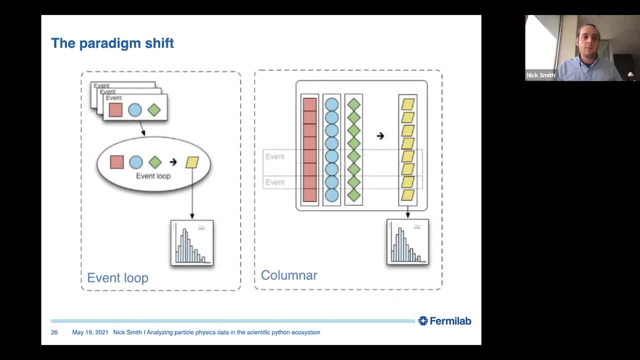 recently is. you know, we've gone from this paradigm of in treating each in the event individually. you know you've always been working in a few different ways, for you know, we've taken the best of the latest well-known algorithms and we've also taken some really interesting models. 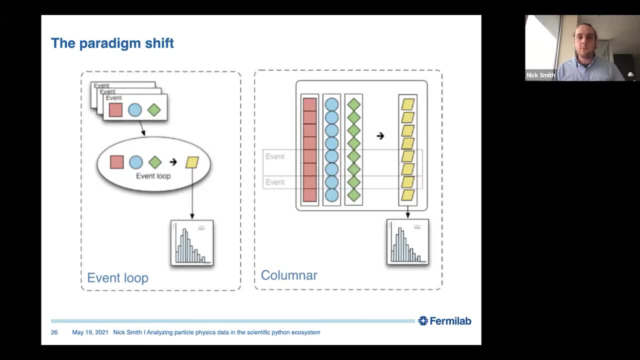 that're in the digital domain and we've taken some really interesting models that are in the data zebrality. but we also did a. we've taken some very, very real world elements, like you know, a so called sophist um, that are in some sort of, you know, mostly c plus plus, but sometimes python. 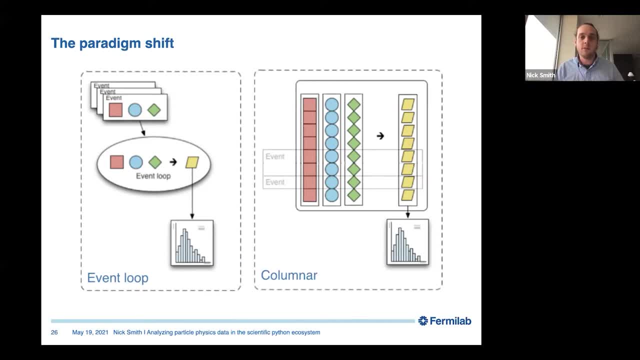 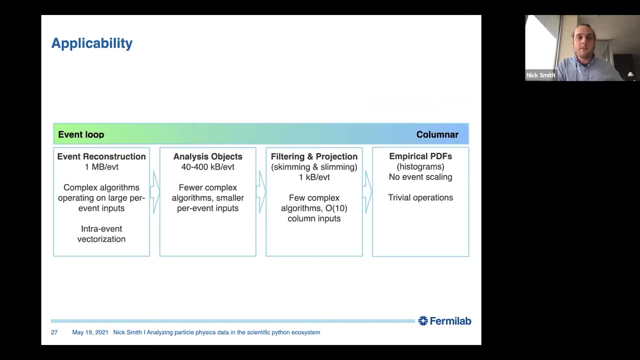 uh event loop code where you would do your different processing and then fill some histograms reasonable to to analyze in in user time and of course it doesn't work all the time right as you get towards the left half of that etl pipeline. event loops are more appropriate because you have 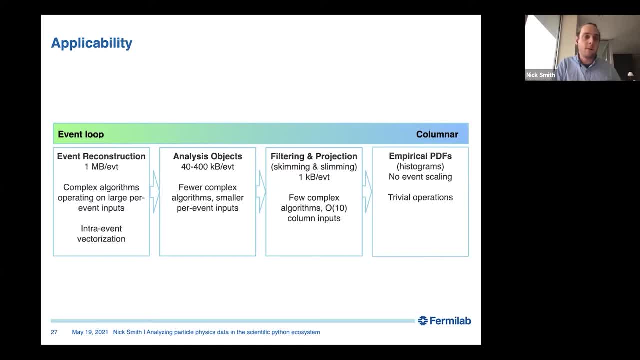 more. you know complex algorithms operating on very large per event input. you know you can even have intra-event vectorization. you know we have 70,000 crystals in our detector. each of them you need to reconstruct the pulse that's. that's paralyzable in of itself. you don't need to. 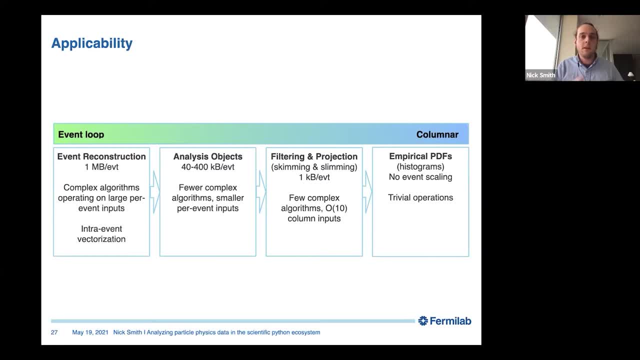 vectorize across events and then you have analysis objects. eventually you start filtering them and projecting, making different, you know composite variables and finally you're operating on histograms which are just numpy arrays at that point. so it's very trivial and it's almost obvious that you want to do something column, right there. the other sort of paradigm shift we're seeing is: 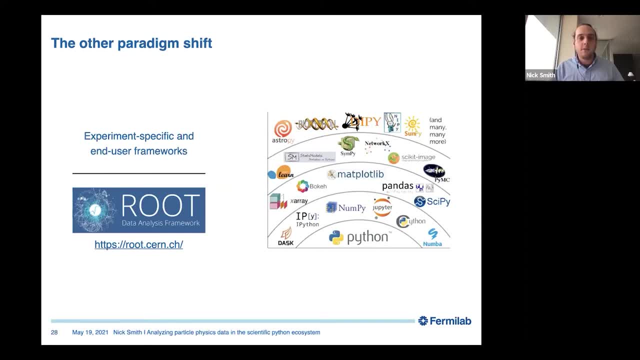 we're moving from these experiment, specific and end-user frameworks based on top of a monolithic code base that was, you know, developed over 30 years, called root, into this sort of software ecosystem where there's an onion of different components, each is targeted on a specific, you know, application, a specific piece of the puzzle. 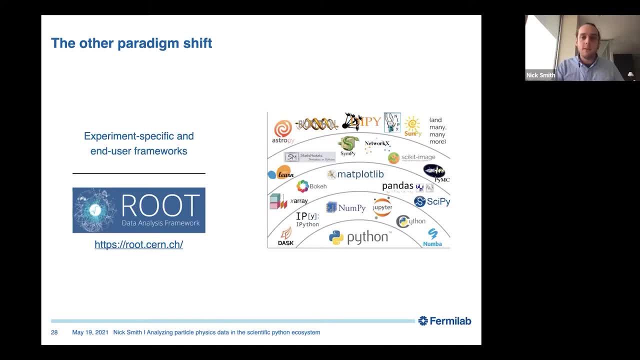 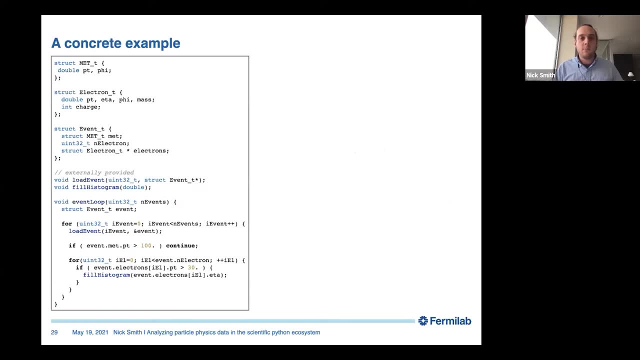 and we're trying to see how we can use these existing pieces and where we need to add our own pieces to make it work. so, to give you kind of concrete example, i've put together this, this c code, that sort of represents, as best i can in a nutshell, some of the problems we ran into as we migrated into this ecosystem, and i'll step 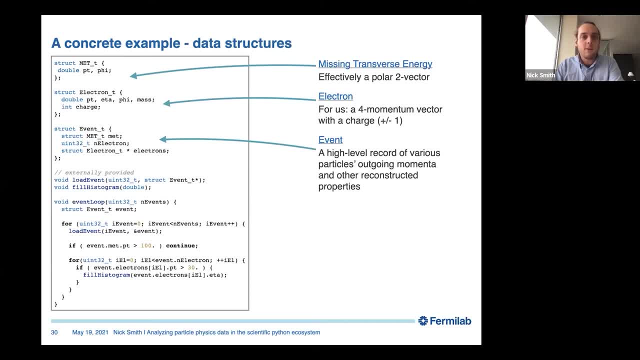 through it, so don't worry about reading it right away. so at the top here i'm defining the data structures. you know we have this thing called missing transverse energy. it's effectively just a two vector with polar coordinates. electron is a four momentum vector, so it's four components. 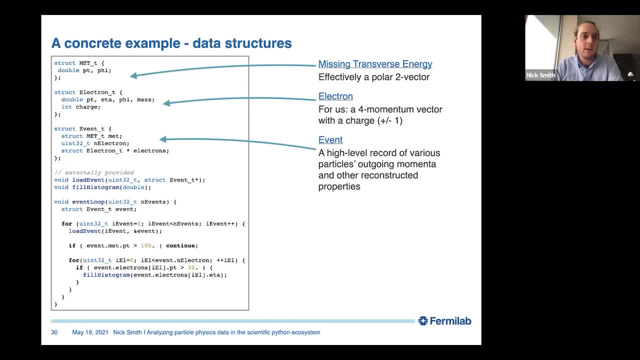 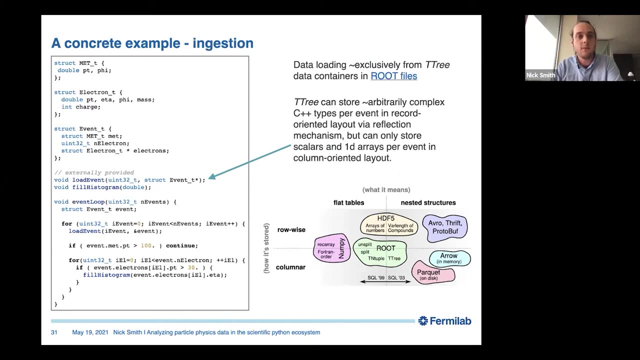 and a charge and the event is just a record that contains, you know, this missing energy value and some number of electrons, various number depending on you know, each collision may produce different number of outgoing electrons. then we have some function, externally provided, that loads this event from some data source, some. 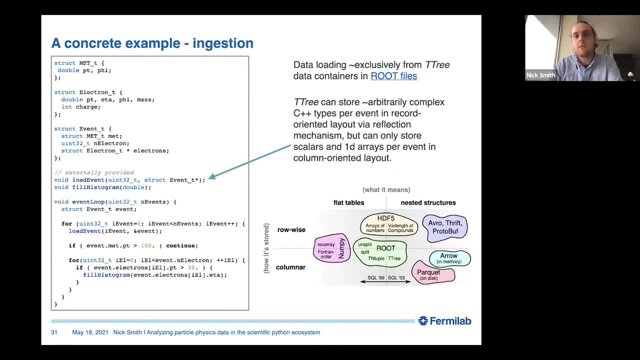 some file and in our field the data is pretty much exclusively loaded from t trees. which are these data containers that were developed in the root ecosystem? the kind of interesting thing about them is they're actually can store arbitrarily complex c plus plus types per event in a record oriented. 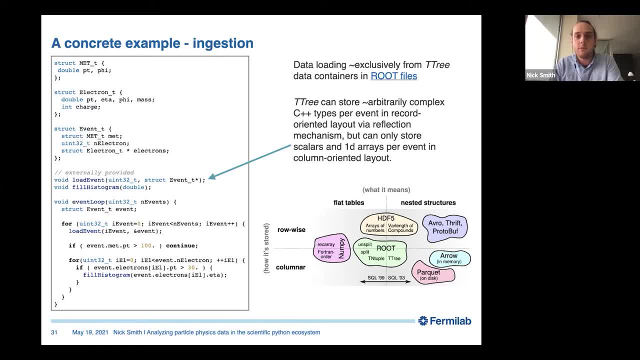 manner because they have this c plus plus reflection manner mechanism. actually, you root has a c plus plus interpreter, which is kind of interesting, but you can only store scalars and 1d arrays per event in this column oriented layout. so it's there's a bit of a impedance mismatch between this, this file type, and the more modern tools. 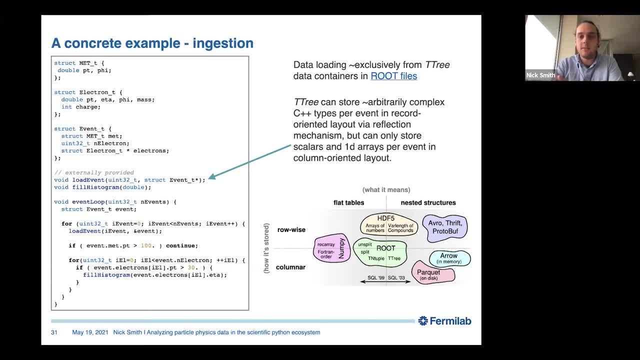 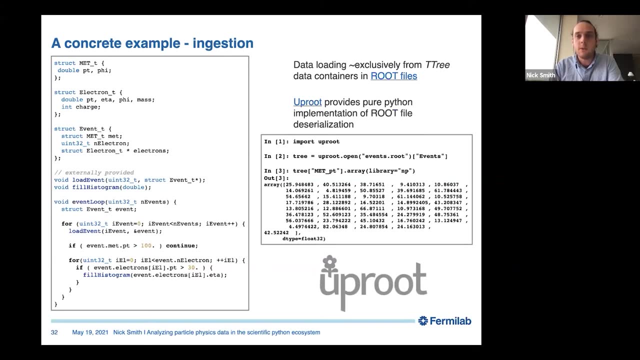 in the more modern data formats like parquet, and so you can see in this diagram kind of how the the t tree lives in this sort of middle ground between very record oriented things like hdf versus very calmer things like parquet. so that's a good thing to keep in mind for that. but nevertheless, you know we developed a tool. 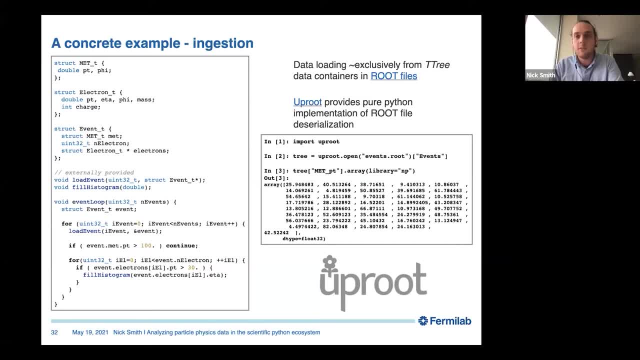 called uproot. that basically provides a pure python implementation of this deserialization so we can open this, this root file, open the events tree and extract numpy arrays. so this is a real missing energy vector values. this is the radial component. we call it pt for reasons i don't want to spend. 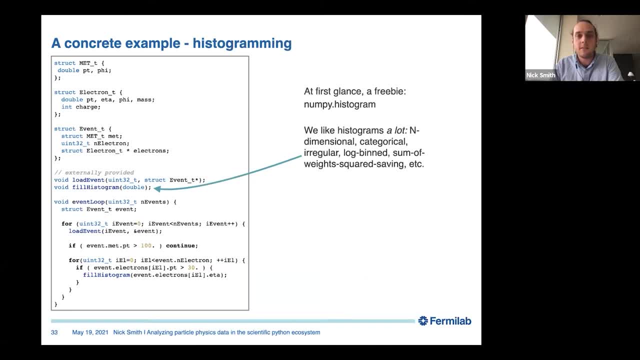 time on. so you know, now we have data access. seems like a freebie, right? We have NumPy histogram. that should be enough, but it turns out Hartfield really, really likes histograms. We like n-dimensional, categorical, irregular log, bin, sum of weight squared. saving all these different things, because histograms are a great. 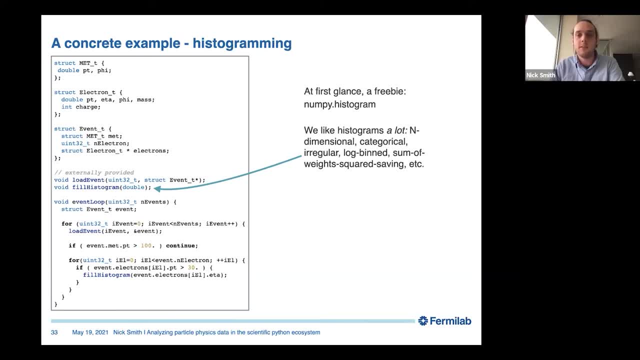 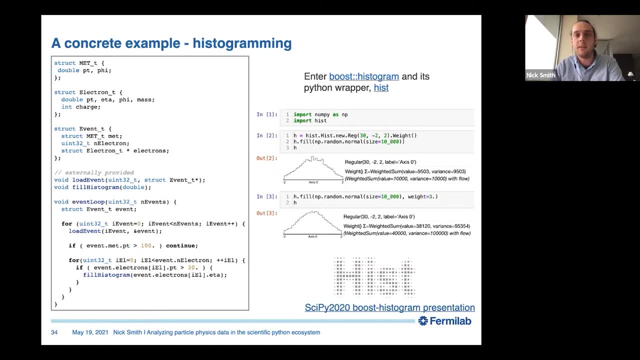 way of forming empirical PDFs. you know well-understood statistical properties from data that is too large to fit in memory, So we have a package for that. Actually, Boost Histogram is a package in the Boost C++ library, and then there's a wrapper called 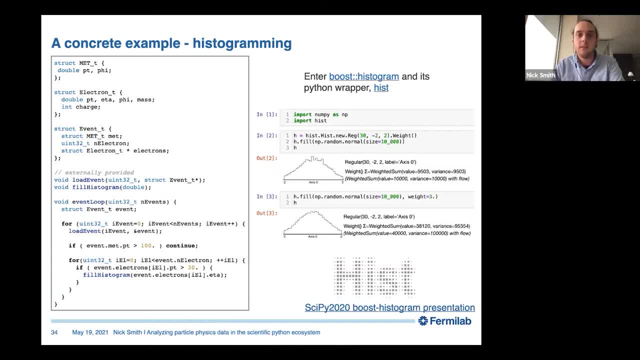 Hist, which lives on top of it. And you can, you know, you see an example here of filling some regular binned axis between negative and two and two with some random numbers, and then you can fill it again with some weight and it stores properly all the. 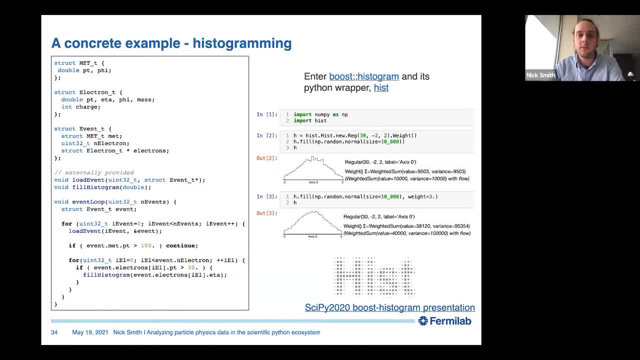 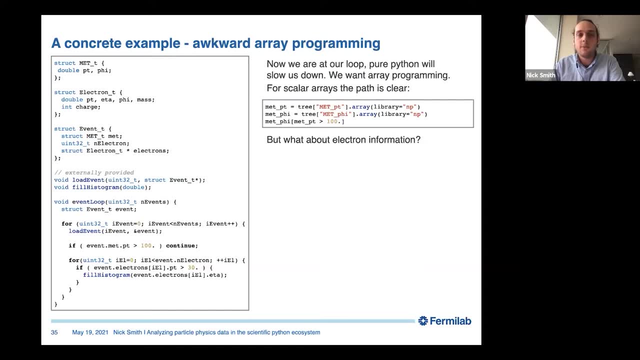 sum of weight squared. so there's statistical information to know that and you can see more at the presentation. And then now we have our event loop and we need to convert this to some sort of columnar, you know vectorized analysis. We can't use pure Python because you know it will slow. 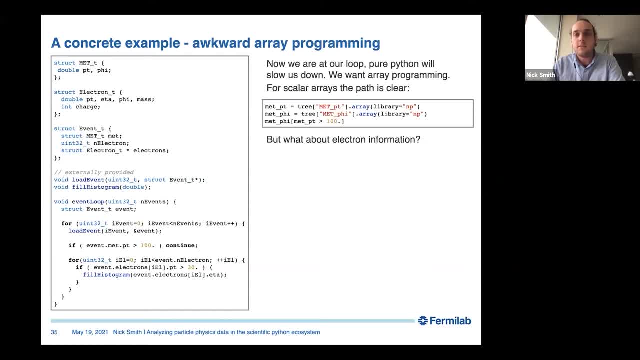 us down too much. We want array programming For scalar arrays. this is mostly clear, right, We? if you just have a numpy array, you have two numpy arrays and you want to look at one after you know filtering on the other, you just use some. you know some fancy indexing, right, But 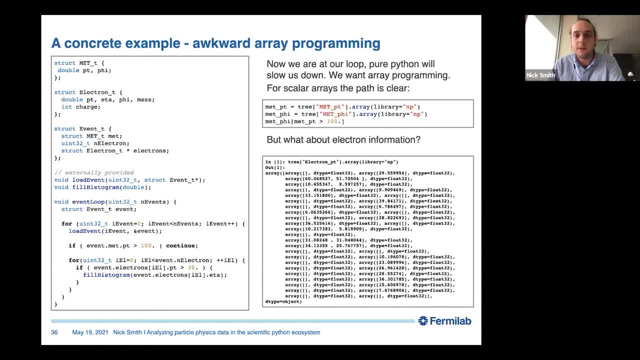 what about the electrons? right, The electrons is an array of arrays and, sure enough, if you try to load that with the numpy arrays, you're going to get a number of arrays and you're going to get an array of arrays, but these are still objects, so you're not getting this vectorized. 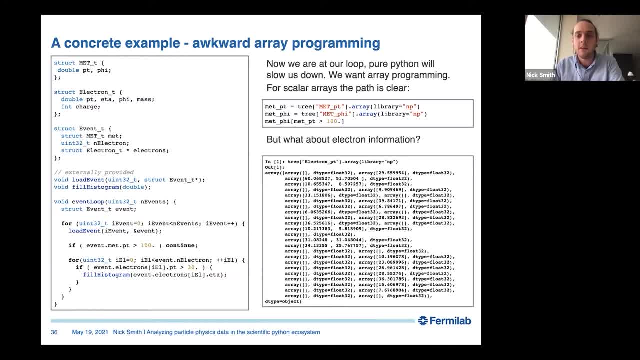 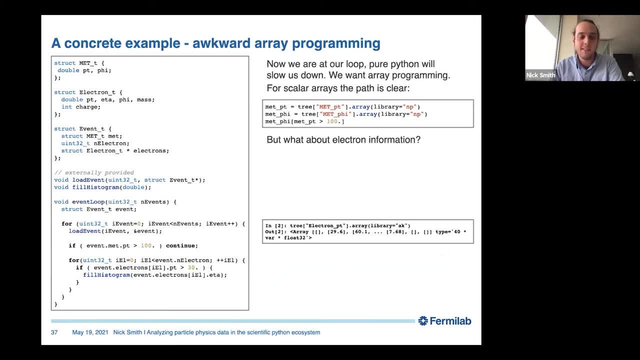 speedup right, You're still operating one per array, So we had to tackle that, and that in itself spawned a huge, huge investment in time, and you end up with this thing called awkward. An awkward array allows you to express these nested arrays, among other things, in a vectorized. 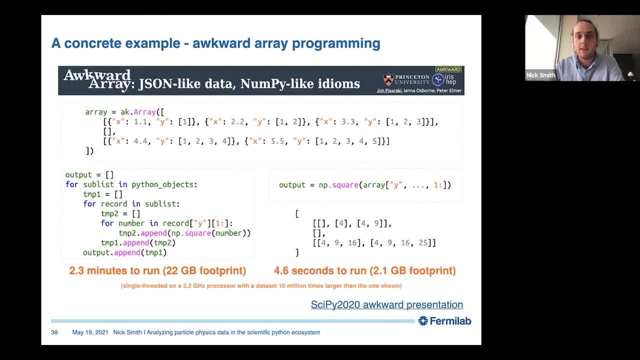 fashion, And you can hear a lot more about this in the SciPy 2020 presentation, but the sort of elevator pitches it's JSON-like data with numpy-like idioms. So you have this natural extension for broadcasting to nested arrays and you also have record arrays, which makes you know. 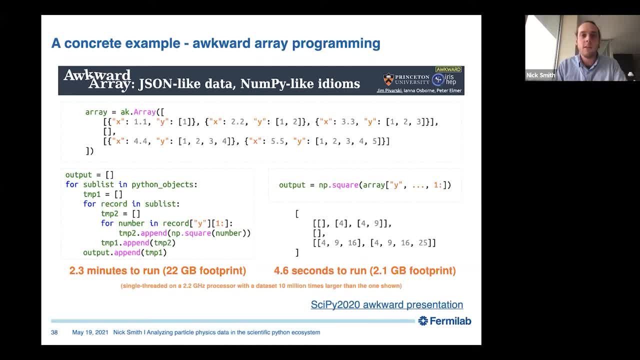 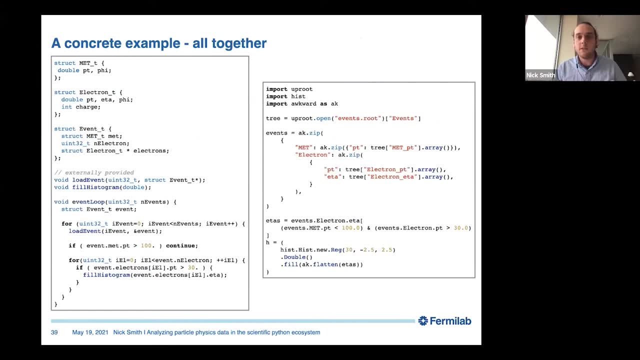 handling these structured objects a little bit easier. So let's put that together. We'll build up our events as an awkward array with some record structure and some jagged structure, and then this whole loop becomes, you know, again, some fancy indexing where you cut on this. 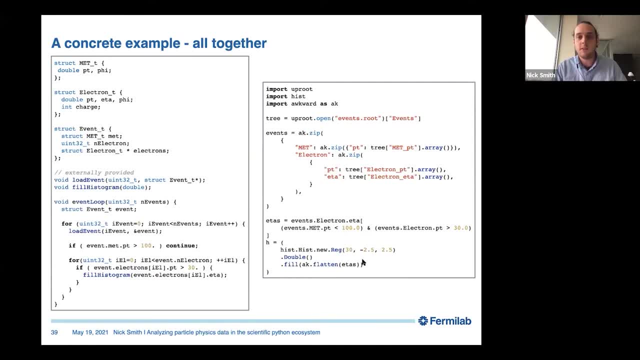 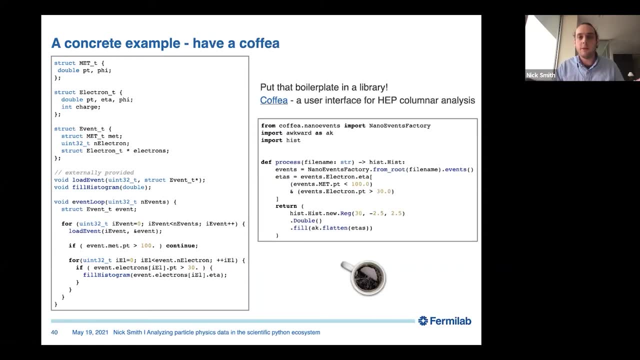 property and then you cut on this property and then you fill the histogram with the flattened, jagged array And of course, you can put all that boilerplate in a library. you end up with this very concise function that reproduces what's done on the left, including the boilerplate that 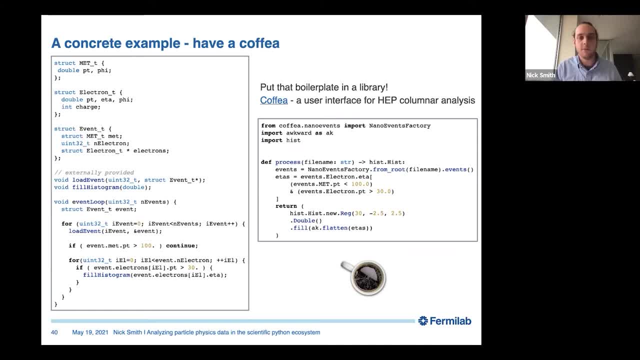 I left out because it was externally provided in the previous implementation. And you know this is nice. We have a scientific Python solution to our, you know, simple problem And so far it's scaled well to more complex problems and we're having a good success in getting adoption with this method of. 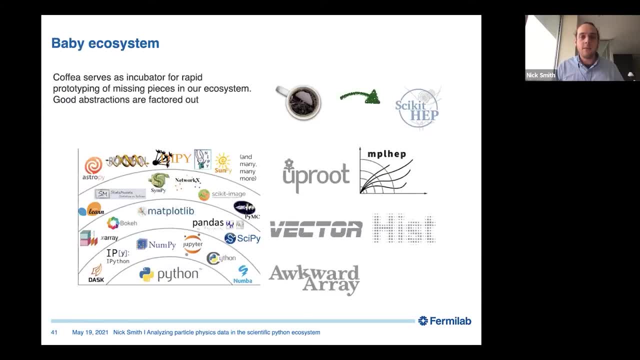 processing, And this, you know, spawned a baby ecosystem of all these different packages that kind of fit in, and we reuse the ones like any ufunc from numpy or SciPy. you know special functions, those we get for free, But then we just have to add a new one, And so you know. 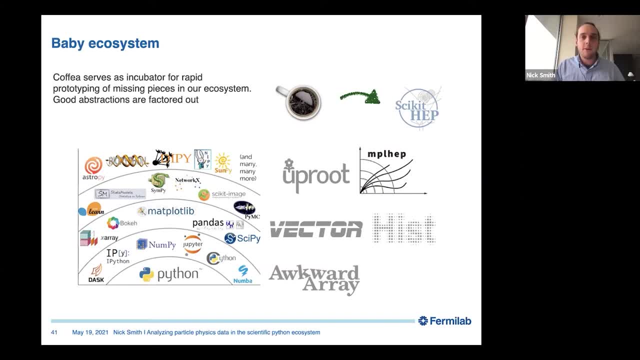 we add a few pieces here and there, And the coffee package that Iksana mentioned this morning serves sort of as an incubator for rapid prototyping for these, and that's what I've been working on with some other people- And then, as we get good abstractions, we try to factor them out or the 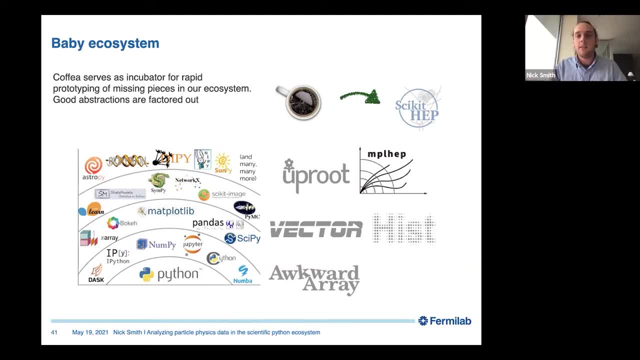 good abstractions may have been found before and they're factored into this sort of scikit-hep meta package. So this is fun and it's nice and you know we've had a lot of success with it And 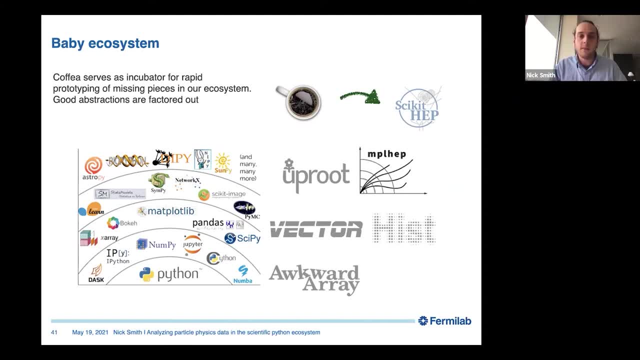 I hope that people here might be able to take advantage of it, and I hope that people here might be able to take advantage of it, and I hope that people here might be able to take advantage of it may look at this package and find success for their data processing needs as well. 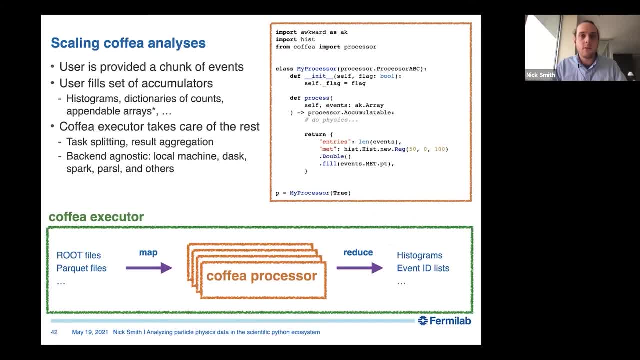 So, and now let's go into scaling. So we wanted to provide a user interface for this, and when we first started, we were still thinking about various backends. So the thing we did is we basically encapsulated all the user code in some sort of class and taught users: just do your. 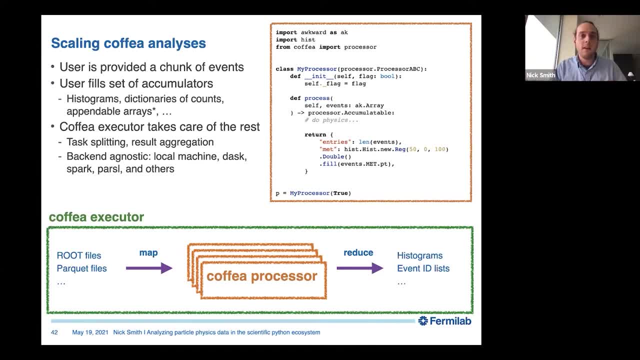 physics in this spot and you know, leave the rest for us. So users fill a set of accumulators, whether that's histograms or dictionaries or Appendable array is not really the best example of a reducible object, right, because it grows every time you append. But people like it. 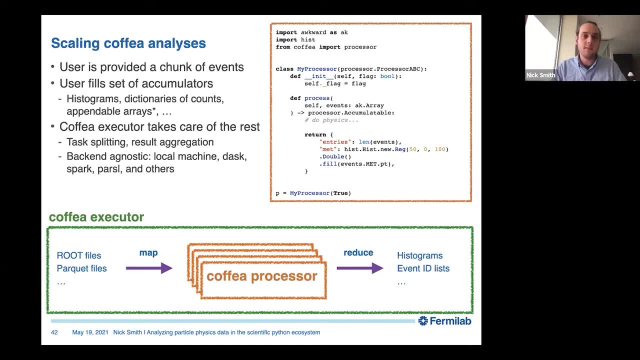 people like to get lists of events so that they can go look at them in the fancy event viewer, like you saw before, And then the executor takes care of the rest. you know splitting the task, aggregating the results. It's basically just one big MapReduce. that's back-end agnostic. 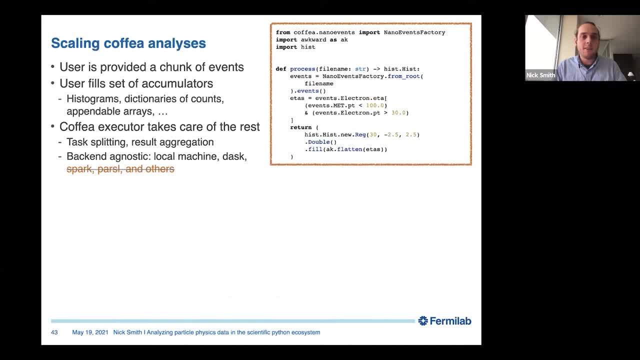 But you can imagine, you know, if I crossed out these others and just left Dask and came back to this example that I was showing earlier, there really isn't much work to be done, right? We just import DaskBag, add and you know. 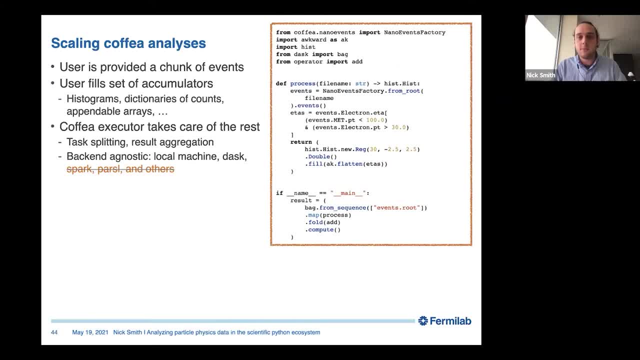 make a sequence of our input files: map the process function and fold with the add operator, and then we're done. So that's great. So, yeah, this is really nice. Our task is very simple: MapReduce. we don't need any operations. 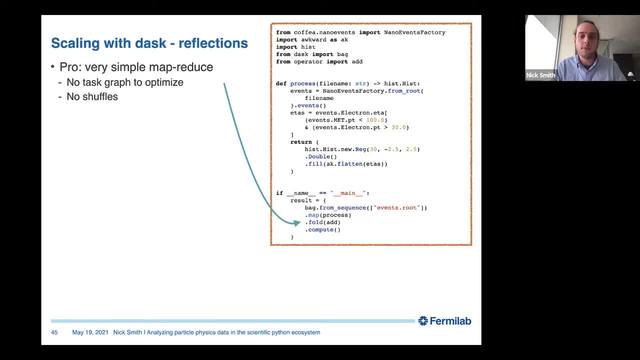 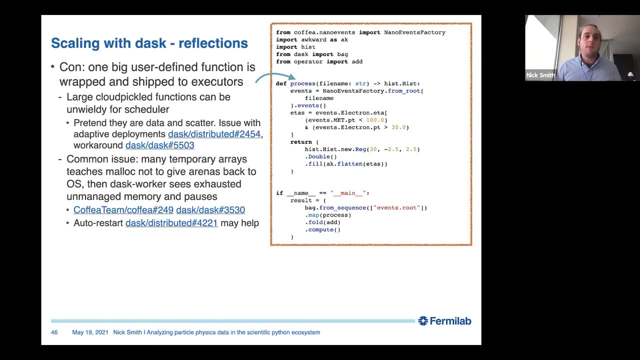 We don't need any optimized task graph, We don't need any shuffles, So that's all very nice. But there are some cons, right, Like we're putting all this, all this processing, in one single user-defined function and we just wrap it up and ship it to the executors. So 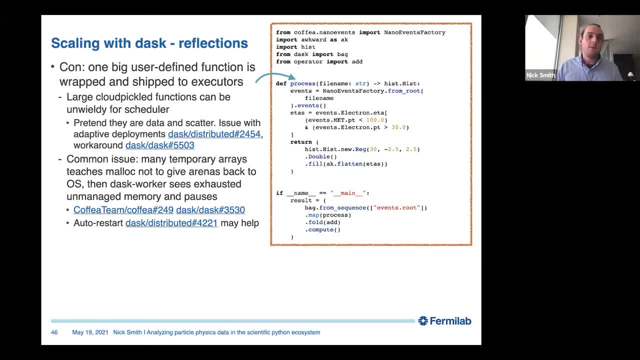 some issues there are going to be. large cloud-pickled functions are hard for the scheduler to handle because they're like you know, these are like multi-megabyte and the scheduler is trying to pass them to all the workers. That's kind of a bottleneck. One solution to that is: 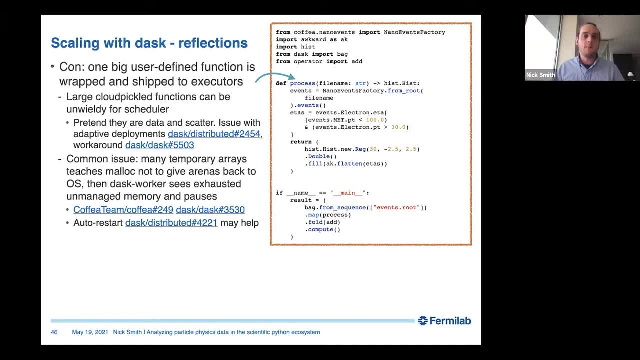 to pretend they're data and scatter them out. So you know we're not going to be able to do that. And then you know, you know, issue a closure later. There's some issues with that that have workarounds. Another common issue is because the user code is all encapsulated and there's no 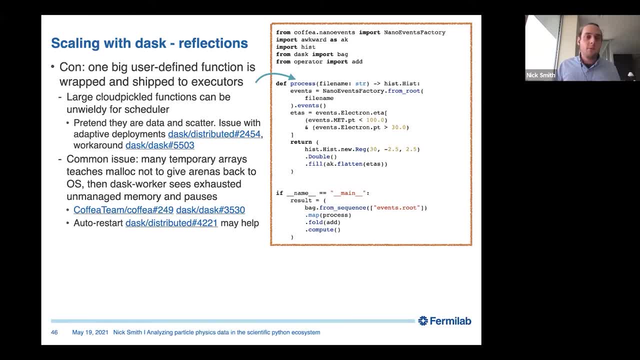 ability for DAS to introspect it. the user may do dumb things. They might make a ton of temporary arrays and run out of memory. or even if they don't run out of memory, they might teach the- you know the underlying C at malloc to keep a bunch of memory arenas around and not give them. 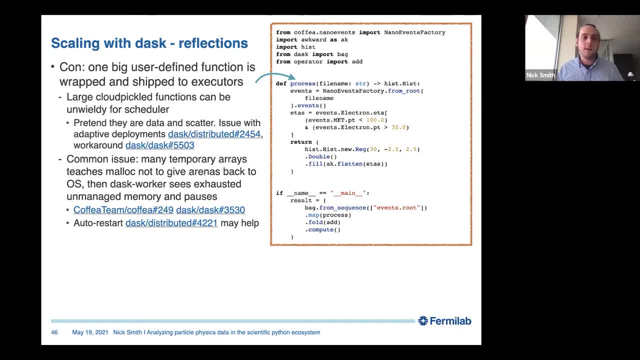 back to the OS. And then you know we're going to have to, you know we're going to have to do the DAS work. that thinks, oh, I'm out of memory, I can't do any more work, So that's another. 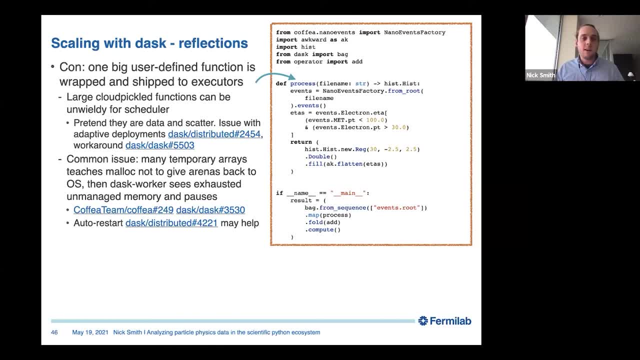 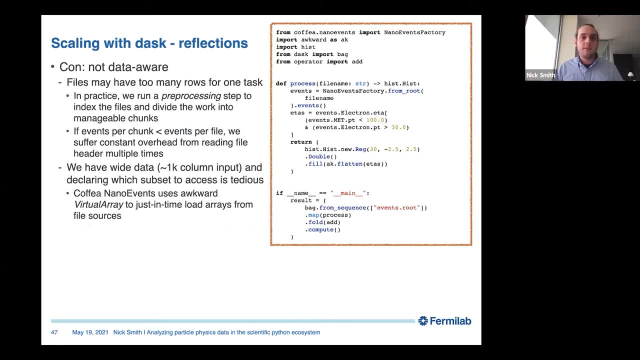 problem that we ran into pretty quickly, But I think there's some pass out of it, including things like auto-restarting from the nanny, The other, you know. the other obvious con is we aren't teaching DAS anything about what the data is. It doesn't even know, It just sees file. 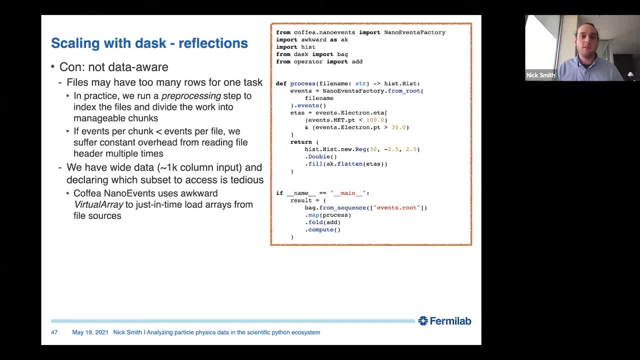 names and you know a fold operation. It doesn't know that there's arrays at all And files may have too many rows for one task, And so you know it's not going to be able to do that. So we have to run the preprocessing step to index the files and, you know, make manageable. 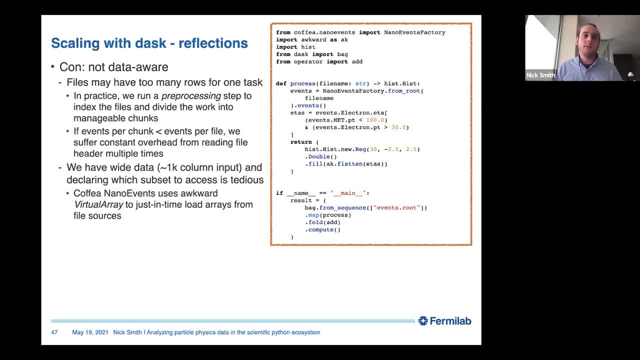 chunks And you can imagine if the events per chunk is much smaller than the events per file. now you have this big overhead from reading the file header over and over again And we have really wide data. We have these sort of distilled information. still has many columns up to a. 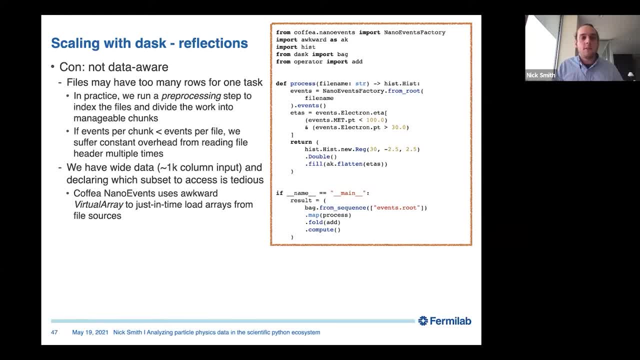 thousand And each person is only going to be interested in some small subset, maybe like 10% of it. So what we did to solve this problem of the boilerplate basically is everything is just-in-time loaded, So when you see this events object being built, actually no arrays are actually read from. 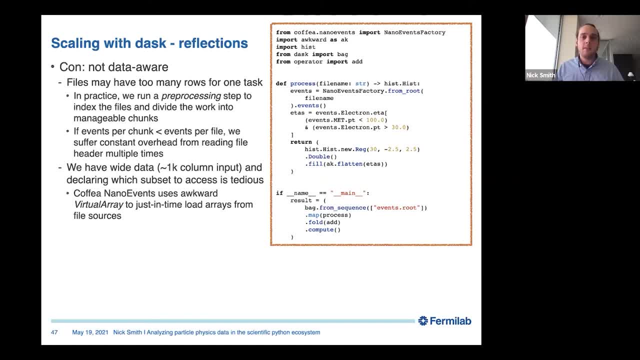 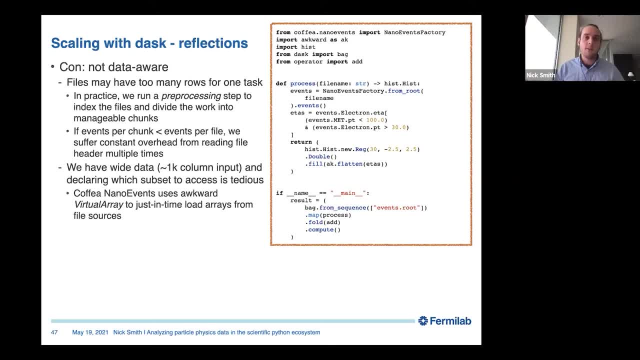 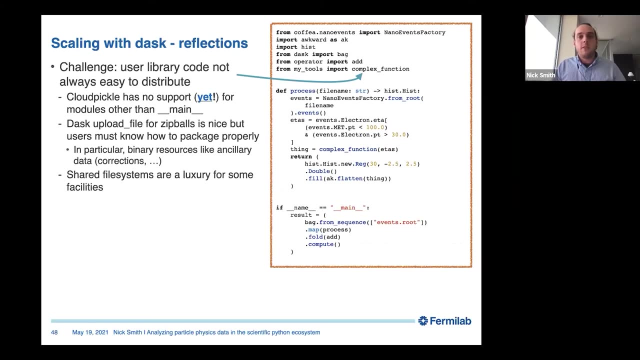 teach the scheduler ahead of time what columns you want to access. You have to define your schema up front. So you know, this is another case where we're probably not using the Dask system to its fullest and we need to find a better way to do it. One other challenge is user library code. You 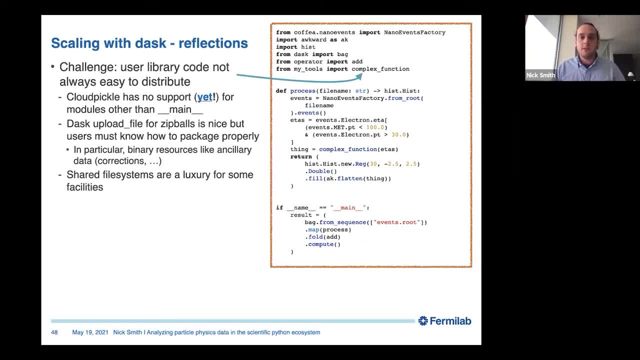 know, if someone comes along and they want to put this complex function in their my tools Python module and import it, it gets to be a pain point. I mean there are solutions like Cloud Pickle is soon going to have some kind of a problem. I mean there are some solutions that are going to have 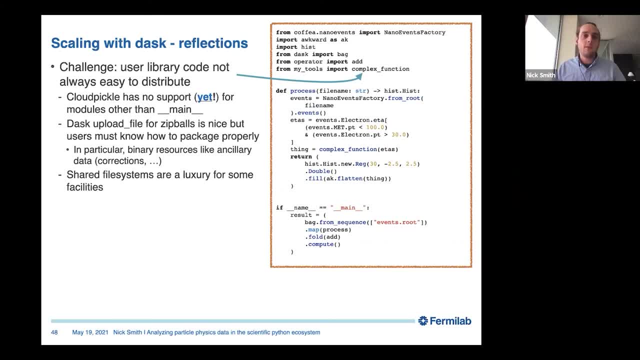 some kind of a problem. I mean, there are some solutions that are going to have some kind of a support for being able to Cloud Pickle modules out of the main, Of course. then you have all the issues with Python versions and all that. Dask has this built-in upload file for zip balls. 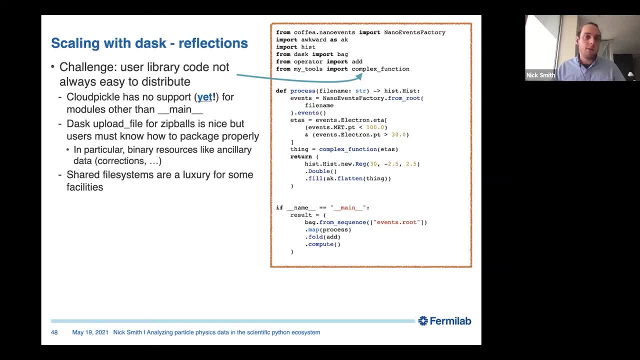 which is very nice because if you make your zip ball properly it will upload it and reload the module in the runtime, which is very slick. But then users have to know how to make a proper Python package, including in particular loading like extra binary resources. Of course some people are. 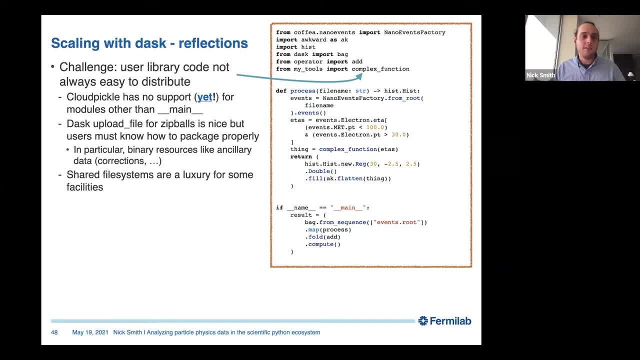 lucky to have shared file systems, and then all of this doesn't matter. You just read your files as if they were running in the same working directory that the client is in, But that's a luxury that not all facilities have. It's a challenge to maintain a distributed shared file system. 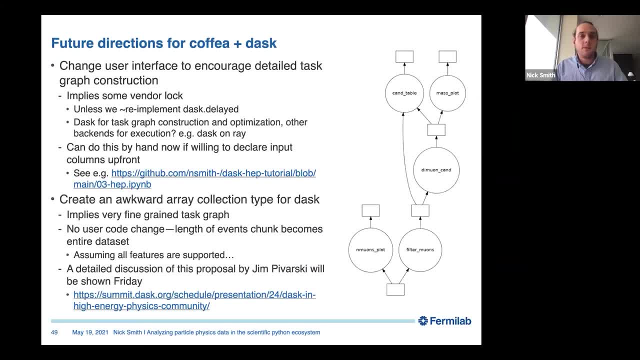 So these are the challenges we saw, and some ways we think we can tackle them include changing the user interface to encourage more detailed task graph construction. So then we need a little vendor lock right. So I don't think we should re-implement Dask Delayed. I think it's. 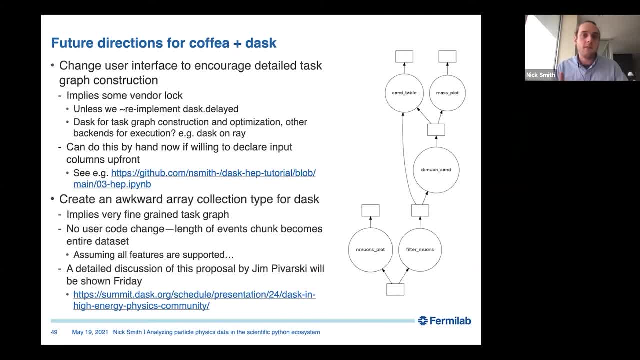 excellent as it is, But that does mean we need to teach the user to make these delayed objects. assemble the task graph or some facet of that, and let Dask go to town optimizing it. And in fact I think I've seen this now, where Dask is used for task graph construction optimization. 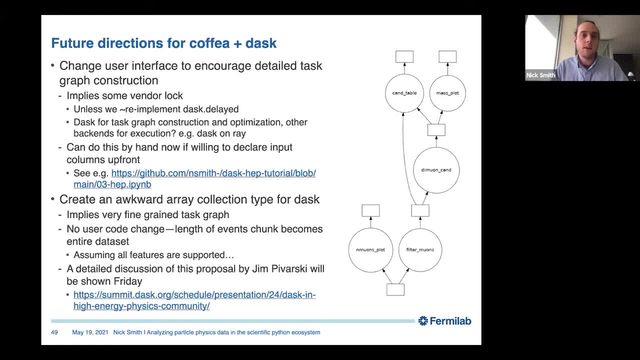 and other backends might be used for execution. like Ray, I think that's a really interesting avenue, because you can think of Dask, as This is one of the pieces that Dask is really providing to the community is this ability to create and manipulate and optimize task graphs. Of course, we can do this by hand now if we're 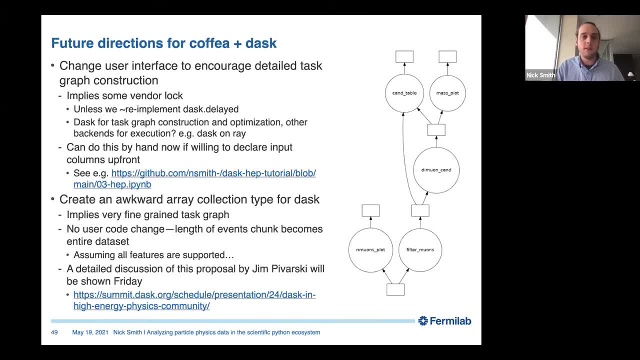 willing to declare the input columns up front, And I have an example of that here in one of the recent tutorials. If you want to go, So that's telling the user to do something. You could also try to go underneath the user and try to trace the operations they're doing through their user. 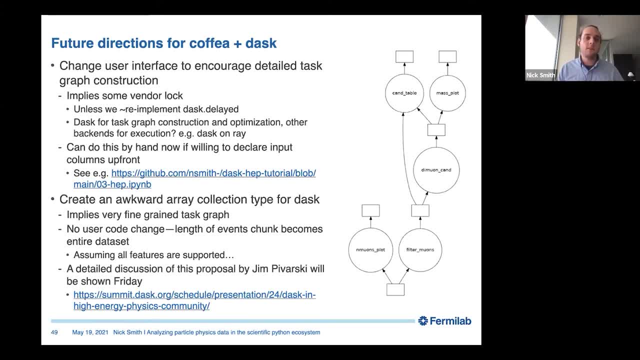 code And then you need basically an operative rate collection type for Dask. So you get a very fine grained task graph, but on the other hand you don't have any user code change, assuming all the features are supported, And you can hear more about that on Friday. 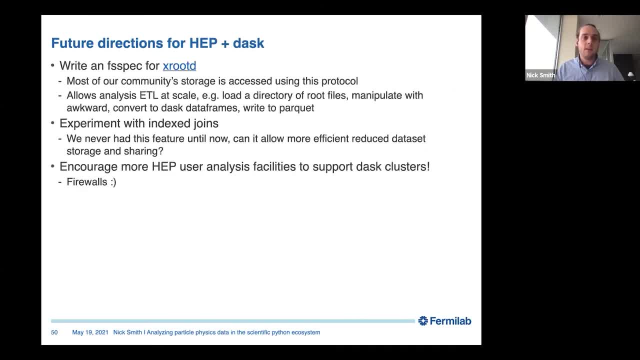 Some other feature directions is Well, as you heard from Oksana this morning, we have our own sort of remote streaming protocol, And FSBEC is a great abstraction for these sorts of protocols. So we should write one for extra D, because then 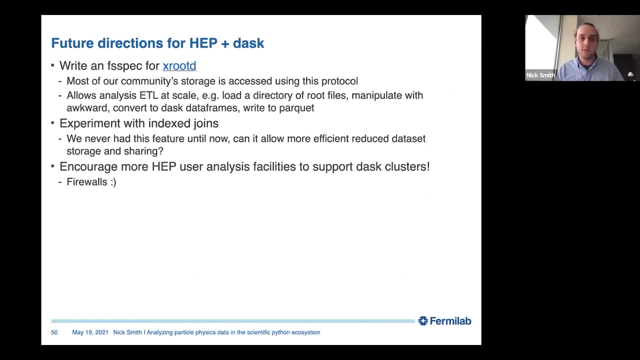 and then, pretty much immediately, we could do all the ETL operations that you're all used to like: loading a directory of root files from S3, manipulating them and throwing them into a data frame and writing to Parquet. We can't do that because we don't use S3, we use extra D. 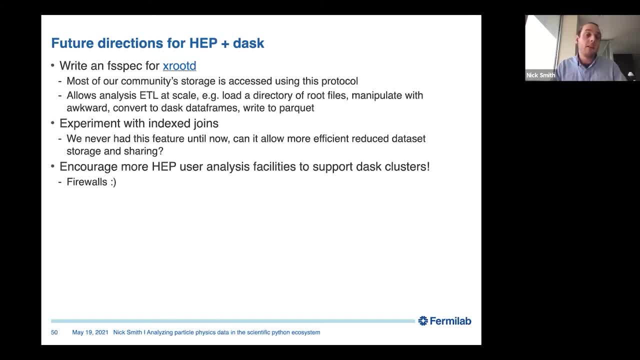 Once we write FSSpec, our life will be much better. I'd really like to experiment with index joins, because that's something we just never had before. You can imagine if two different analysis groups were making different filters, different filtered, distilled data sets. 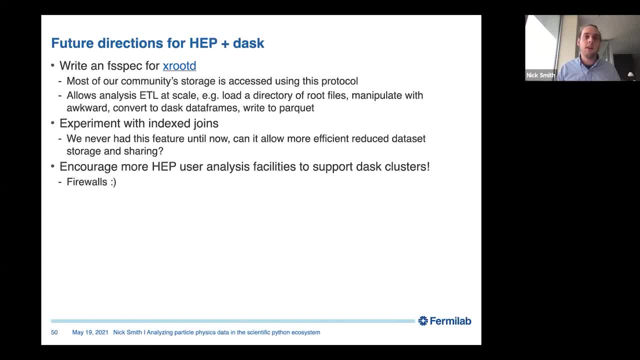 and they wanted to compare some subset of the features from each other. Right now they really don't have any mechanism to. they have to sort of join up manually by the event ID, things like basically dumping to CSV some small subset of them and comparing. 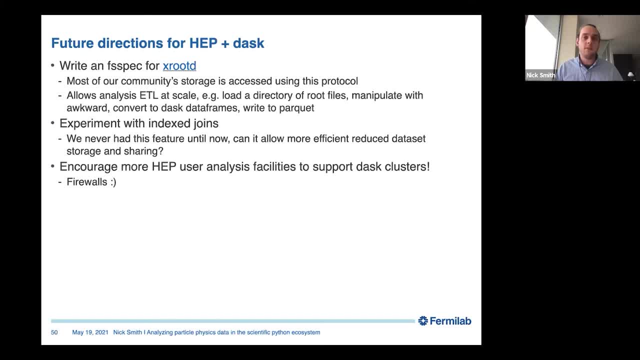 But with the ability to convert into a giant out of memory DAS data frame, you could do joins on the whole data set and that may allow more efficient reduced data sets storage. And last but not least is we need to encourage more hip users. 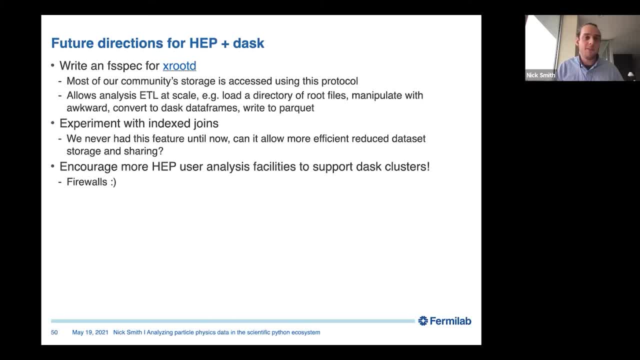 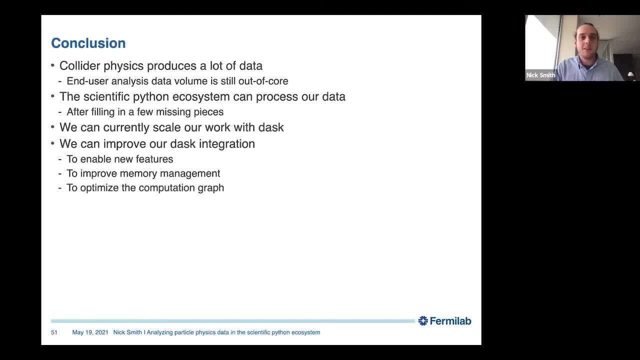 We need more analysis facilities to support these, and that's things as simple as firewalls. so, In conclusion, Collider Physics produces a lot of data. The end user analysis data volume is still out, of course, So it's still sort of of interest. 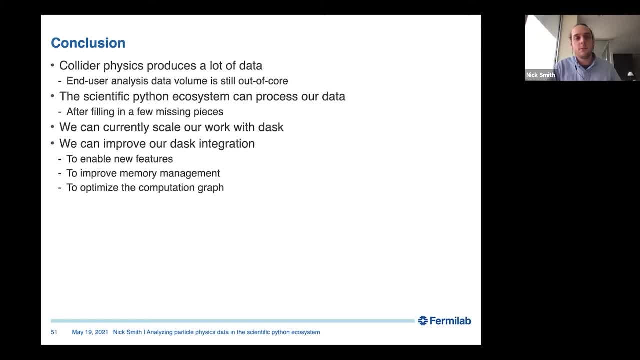 to these distributed systems. The scientific Python ecosystem can process our data after filling in some missing pieces, And we can scale our work with DASC, And I think there's a lot of avenues for improvement that we're excited to start working on and collaborate with the community on. 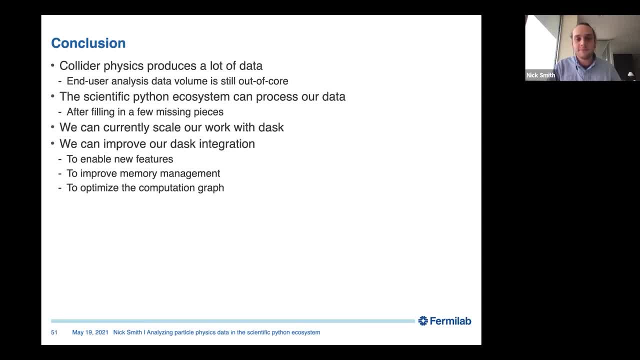 So that's all I have. Okay, thanks a lot, Nick. So we definitely have some time for questions, and there is one in the chat right now. So Thomas asks: is it possible to wrap awkward arrays in X array objects? That's an interesting question. 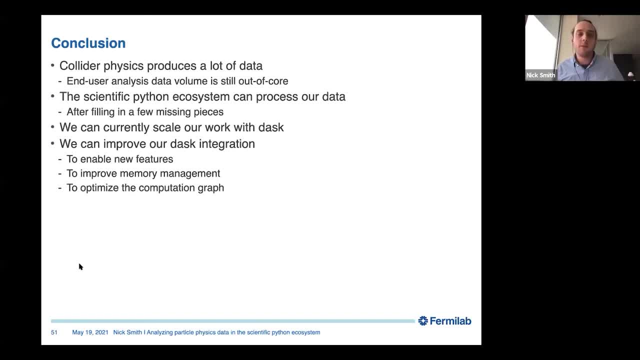 I don't think yet there's an interface between awkward and X array, but there is some work in that direction. Some of the X array developers are aware of awkward and starting to look into it, And I guess there what you're looking for is a feature. 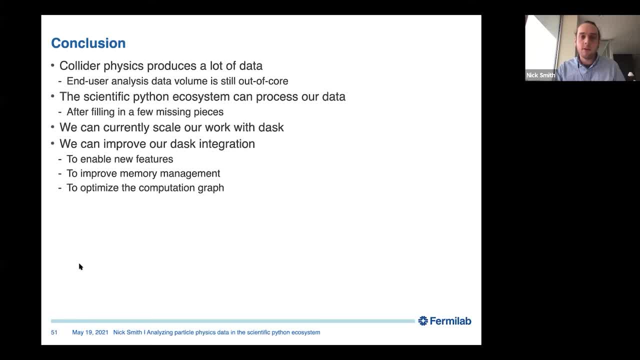 of sort of metadata associated with columns, right I assume, And that's sort of a good motivator for an X array awkward integration And I think that's in the future. So I think that's a good motivator for some of those things. 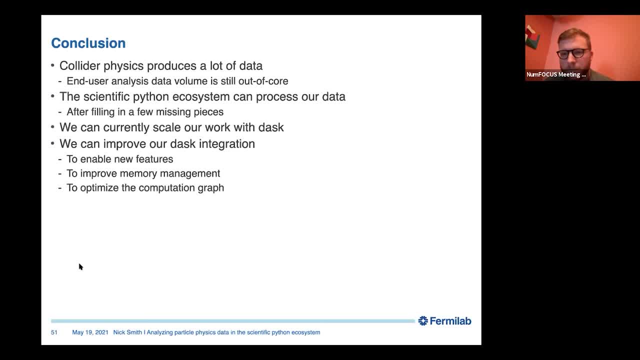 So I think that's a good motivator for some of those things. Cool. so we have another comment from Florian for improved memory management. Don't miss tomorrow's talk. Okay, thanks, Florian for plugging a talk that will be coming up later in the summit schedule. 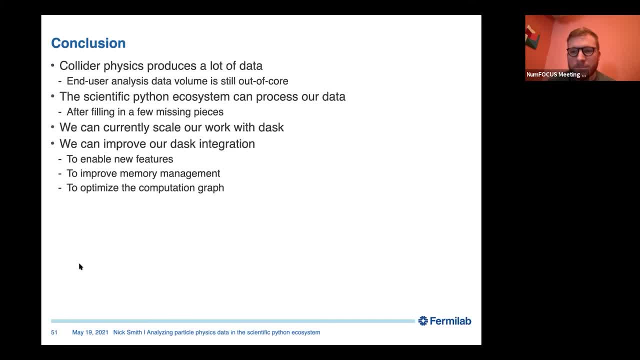 So we still have some more time for a couple more questions. In the meantime, I have a quick question And while there's nothing pending in the chat, you mentioned, Nick, that there's kind of this shift from the upstream to downstream end user analysis. 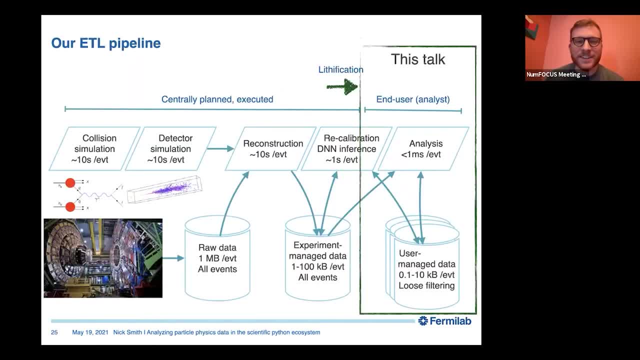 where you bring in Dask kind of in the end user thing part of the story. The question I have is: do you or anyone in the community envision tools like Dask moving upstream at all, Or do you think it will always? will it always be disconnected from that? 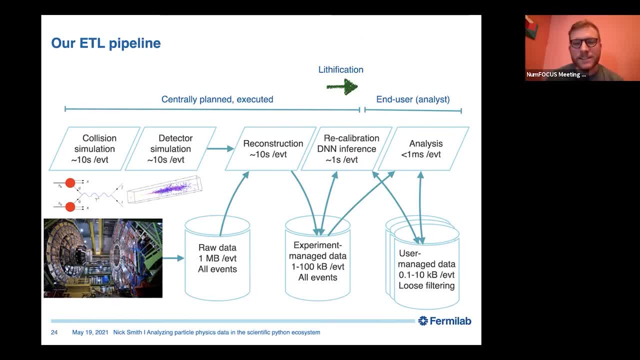 That will always require custom, very domain specific things. compared to to. That's a good question. So I think in principle there's no technical barrier to having tools like Dask run on all tens of petabytes of information. I think it's more just a matter of developer effort. 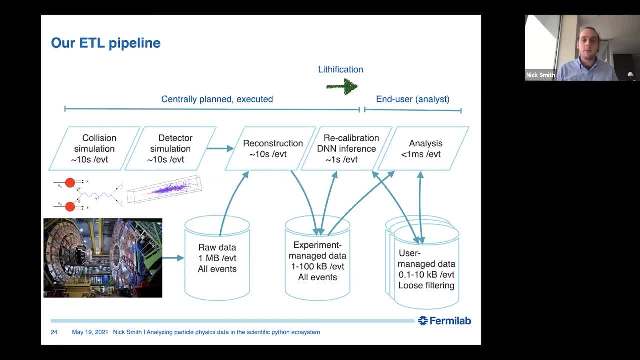 because we have a lot of legacy algorithms written in millions of lines of C++ code And so the students, everybody who comes in, we know that right. the expense- developer expense- of having to port that code to sort of a vectorized 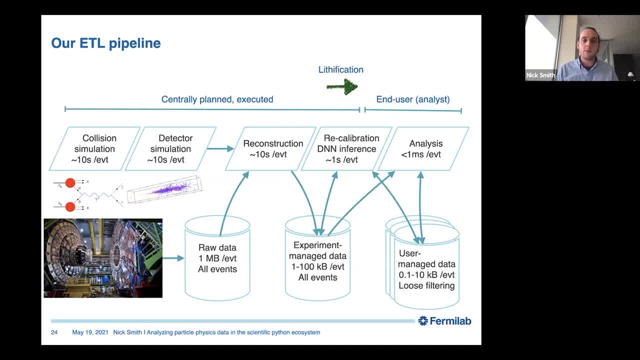 scientific Python is probably out of scope And anyway, I think the improvements that you would see from that are limited up to some level, right, Basically. the further you slide back on this, the less likely you're going to see improvements from vectorizing intervent And since our whole. 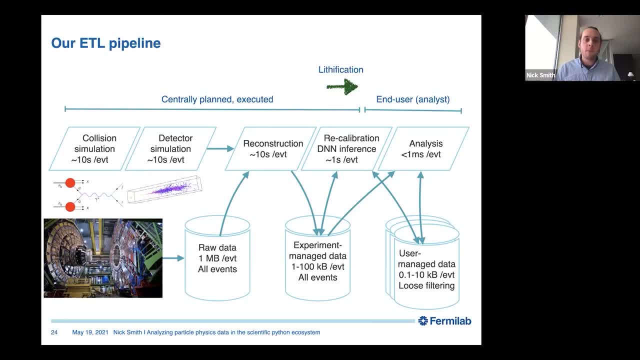 and our whole operation is very. some people call it pleasingly parallel, others call it embarrassingly parallel. Each event is statistically independent, so you can analyze them in isolation upstream. So without the need for these sort of shuffle across join features, there's not a huge motivation for moving it back up the stack, It's just very nice at the 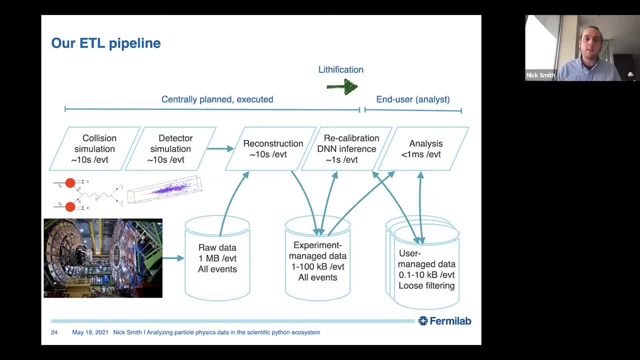 end user level, because it provides a level of interactivity that we can't develop ourselves. We have- you know, you can imagine- with this much work to do. we have our own custom workflow management solutions and they're not. they just operate on a different time scale. They operate. 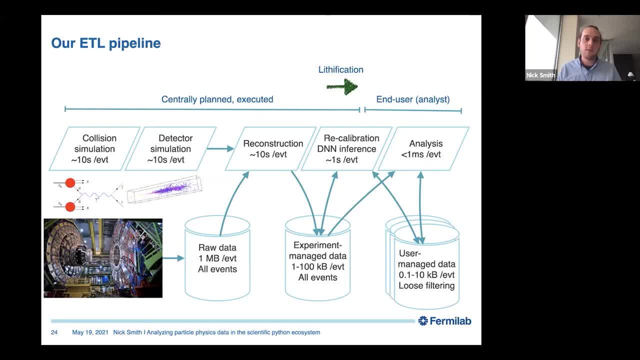 on the hours, hours, time scale, whereas Dask operates on the millisecond scale in terms of task, you know, life cycle. So, yeah, this is different, I think, domains. but you can imagine moving this, this slider further to the left as we find more reasons to go lower level, right with Dask. 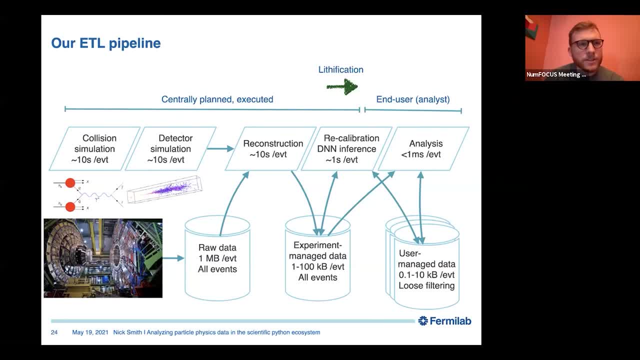 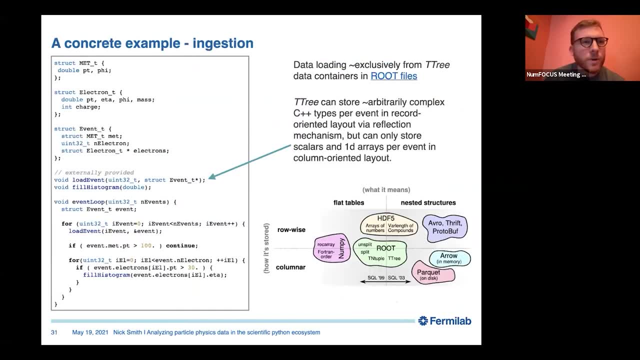 Cool, thanks. We have another question here in the Q&A from Adam You showed a 2D plot comparing HDF5, Root, NumPy, Parquet, etc. Where do awkward arrays belong in that plot? Do they belong in that? 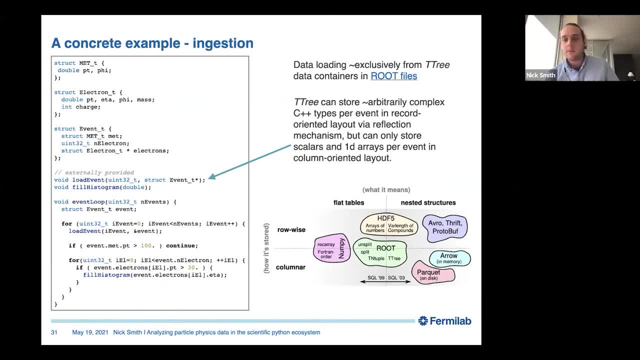 plot at all. Yeah, so this plot is for, say you know, on-disk serialization. although I guess Arrow is in memory And Arrow and Awkward are almost an overlapping diagram, I would say There are a few subtle differences between. 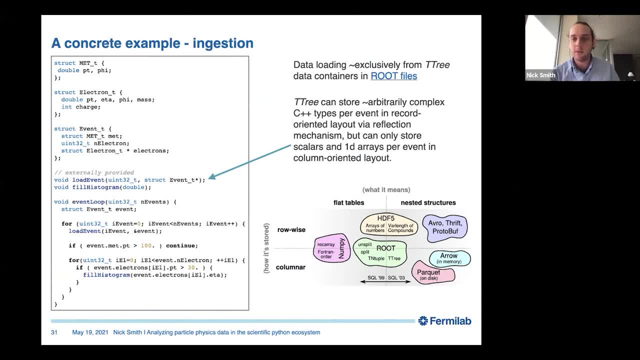 Arrow in memory layout and Awkward in memory layout. Actually Awkward, I believe, is a superset, But yeah, they both sort of live in memory and they both, you know, are fully columnar and they're very aligned. You know, in fact, Awkward could take. 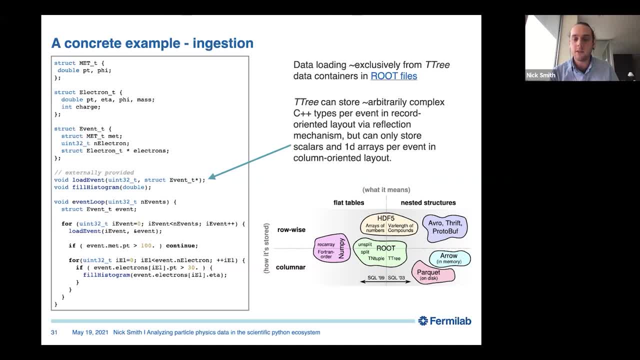 advantage of some of the Arrow extensions, like Arrow dataset or Gandiva or Gandiva- I'm not sure how to say it- And I think that'll be interesting. you know, use things that read Arrow and use the predicate pushdown that these Gandiva library and such provide And then use Awkward at. 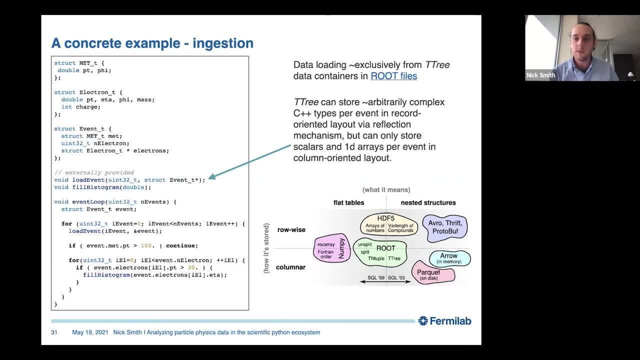 the top level for the things that are out of scope for the community. that Arrow addresses things like these, Something I haven't shown here, but we do need to do combinatorics. So, like you know, take n electrons, choose three or choose two, and consider the properties of that combination. 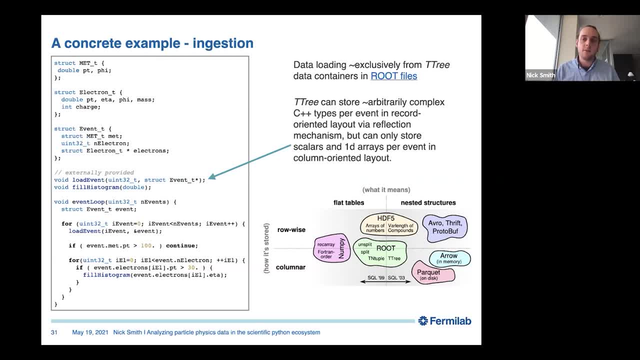 And so that's something that's built into Awkward. that is sort of out of scope for Arrow Great. Any more final questions. We have about one more minute until the next talk, So I'll just remind everyone again that, of course, during the conference, after the session, 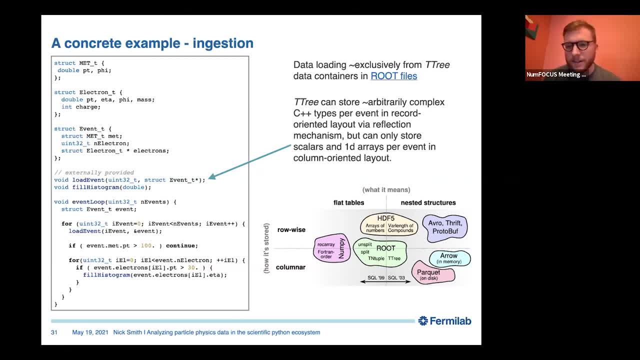 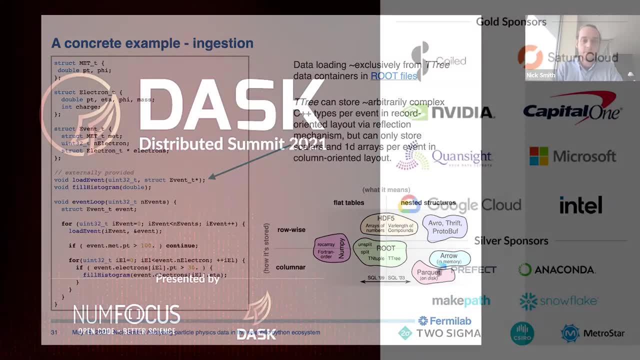 there will be some hangout time in Gather Town and there's no more questions. Thank you again, Nick, for this great talk. Yeah, thank you. Thank you for recording.